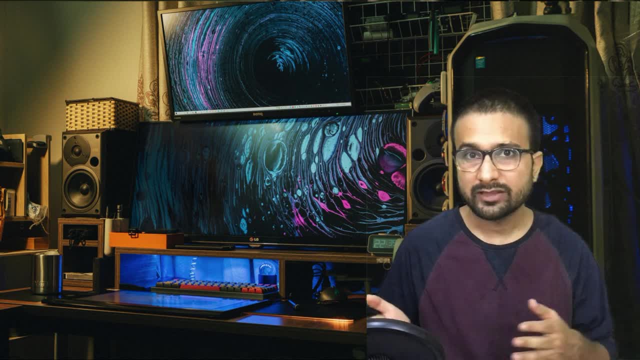 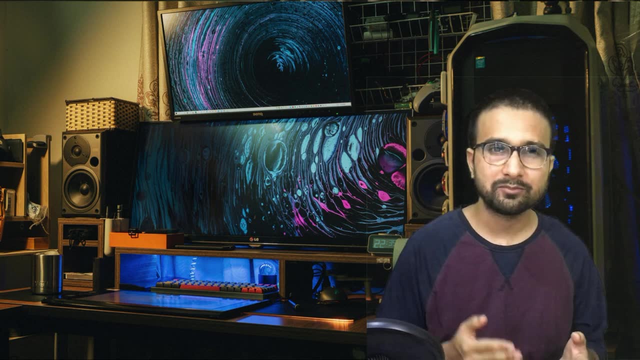 inference, or create a live website with the model running on background and guys. it's a big request to you to please subscribe this channel, because creating up this one hour two hours long free contains consumes a lot of amount of my time. so if you like to support this effort and want me to come up with new, 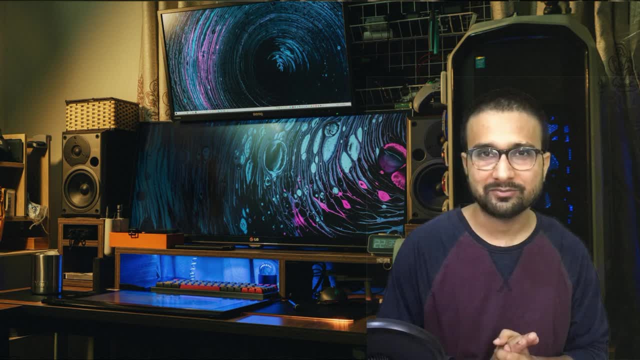 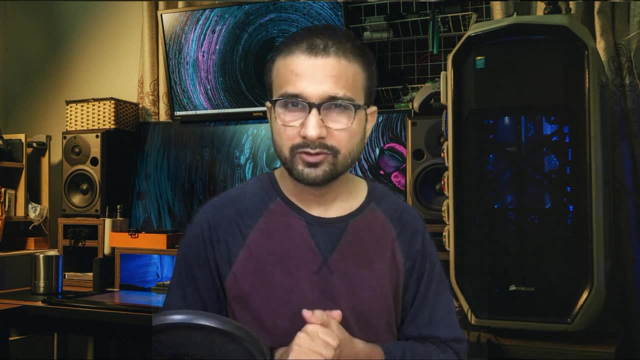 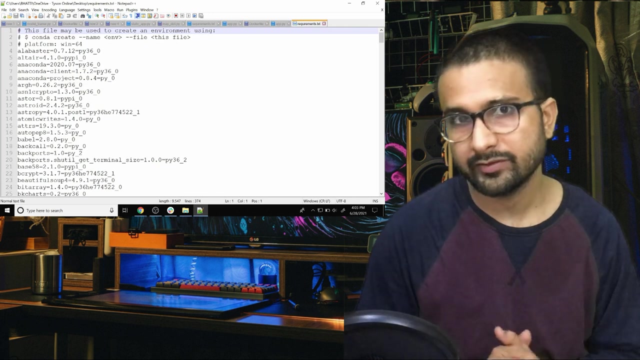 content like this. don't forget to press the subscribe button, guys. so now, without wasting any single moment of time, let's start now, guys, before we start, I want to make sure that you won't face any error because of the environments, because I have seen you asking many questions on my comment section saying that I am 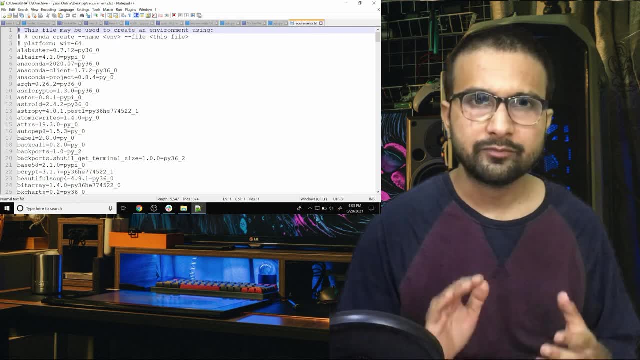 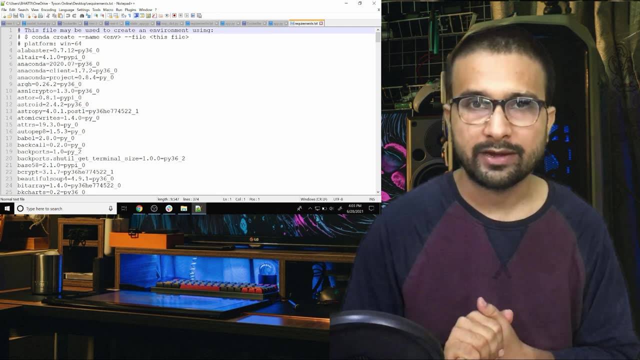 having that environment issue, this environment issue. so what I have done, I have uploaded this complete environment list on the github link and I have provided the link to the github link and I have provided the link to the github link in the description for both this environment and the data set. I am going 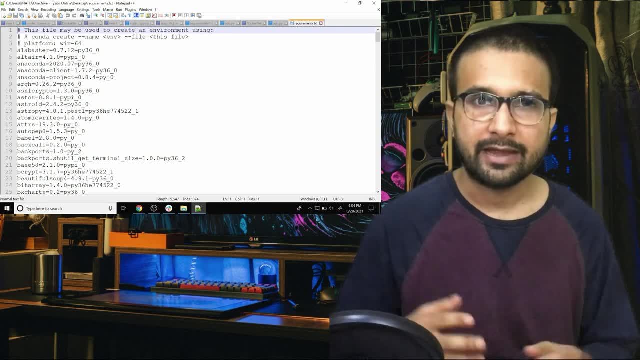 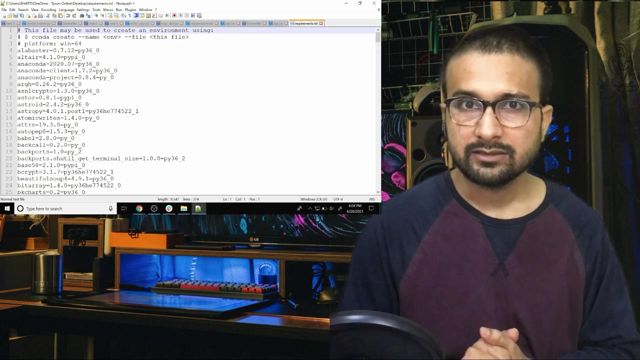 to use. so directly go to the description and download the data set and if you face any errors, go to this github link and you will get this file over there. just check that the environment that I am using right now is having the similar packets with your environment, if you are having any type of environment related. 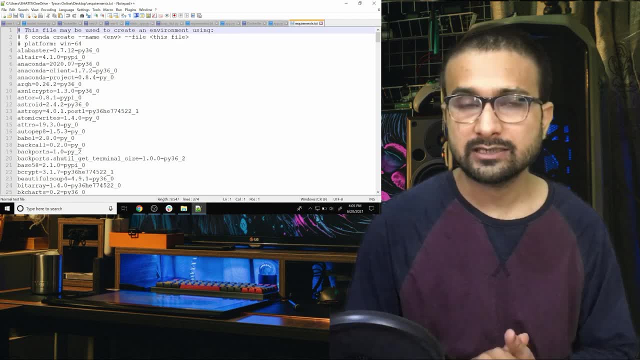 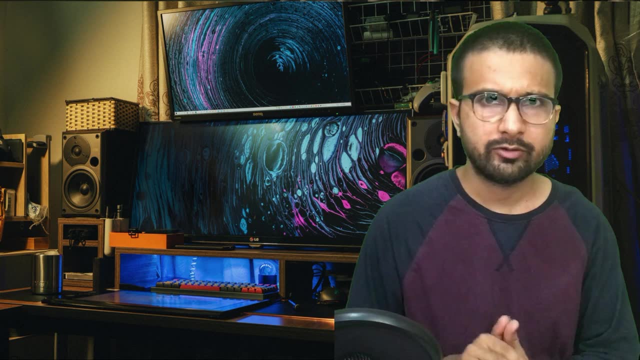 issues going ahead. we are going to talk about leadership scrutiny on github project information as an organization perspective, about github, the data set with us and how we are going to utilize that data set. now, guys, before we jump into our Jupyter notebook and start the coding, let's have a look. 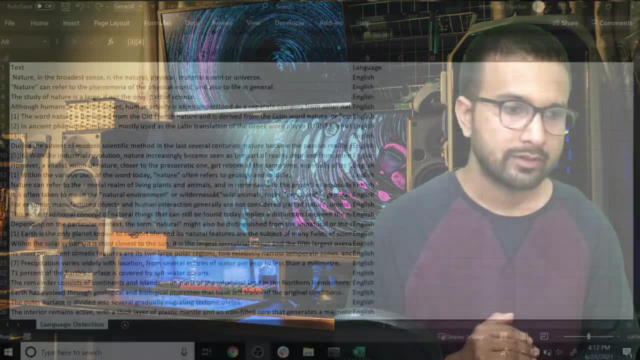 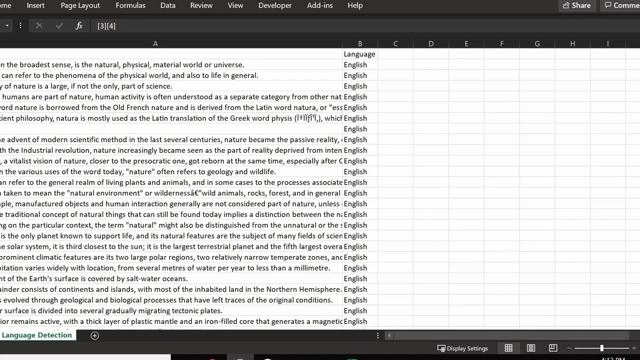 on the data set that we have just now downloaded. so it's a language detection data set and you have text on one column and on the other column you have the language name. this is a pretty good data set because you have every single sentence. I think this is coming from Twitter. it's also labeled for that. 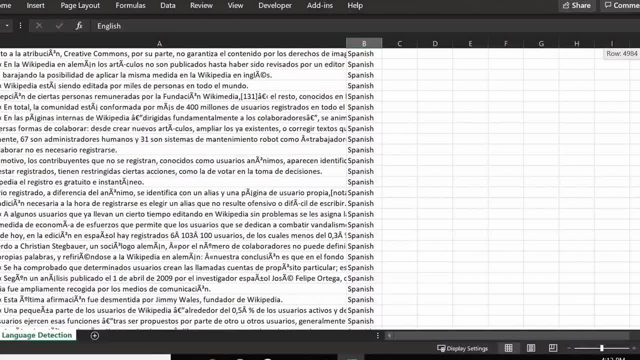 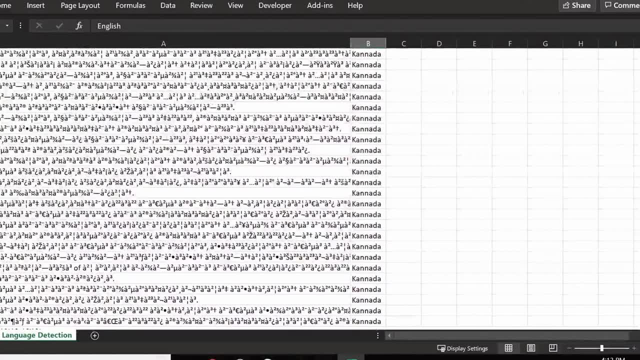 language and if you scroll down with this data set, you will figure out that it has Spanish, it has Dutch, it has French, it has Malayalam, it has Portuguese, it has Kannada and many other languages- I think Hindi also. so around seven or eight languages are there within this data set and we are going to 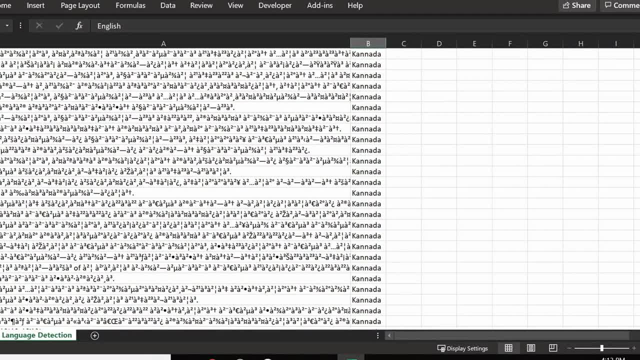 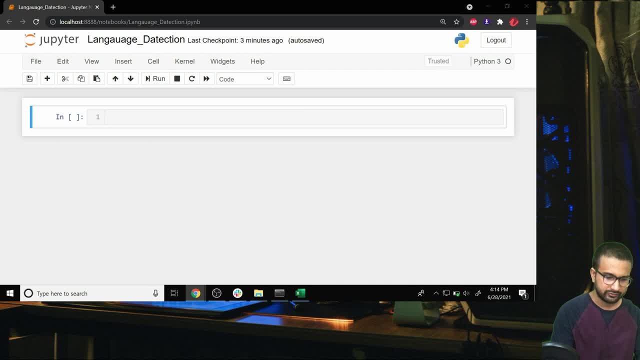 use the Jupyter notebook and we are going to use the Jupyter notebook to this data set to create or to train up the model. so here we are on our Jupyter notebook. I'm going to import some basic libraries like string, because this data set is not clean. we have to do a lot of cleaning, step by step, and these are some. 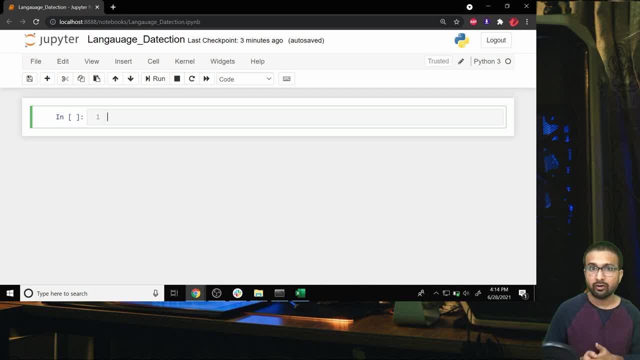 basic, fundamental steps when you that you need to follow whenever you are going ahead on a project based on NLP, and these are very foundational concept like cleaning and coding and so on- by cleaning up, stop words and all, and I'll show you how you can do it with. 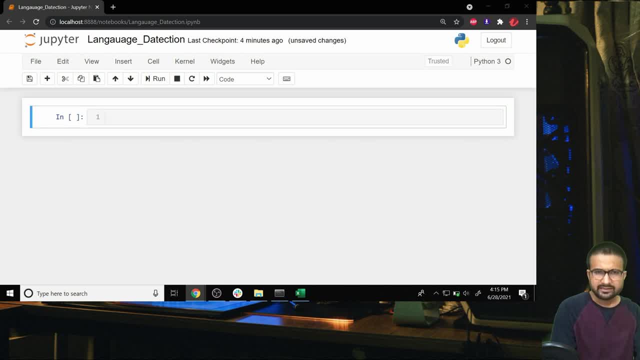 simple code. so, guys, let's import some basic libraries which are required for any NLP project. so let's import string now pandas, numpy and we'll need re, and Then we need to plot also. So we'll need matplotlib and we'll need seaborn also. 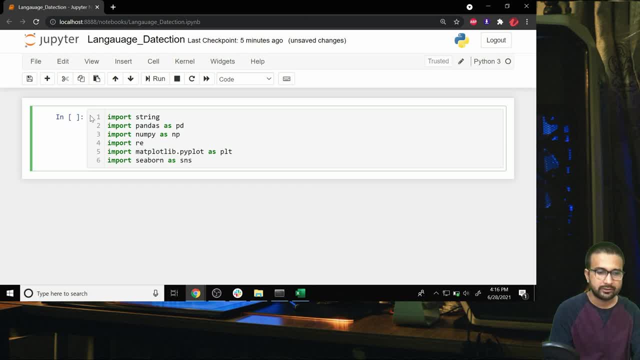 So let's import these libraries based on need. we will keep on importing other libraries, So I'm going to run this. So, first of all, we'll start reading up this dataset And since I've already saved this dataset within the same folder, so I do not have to. 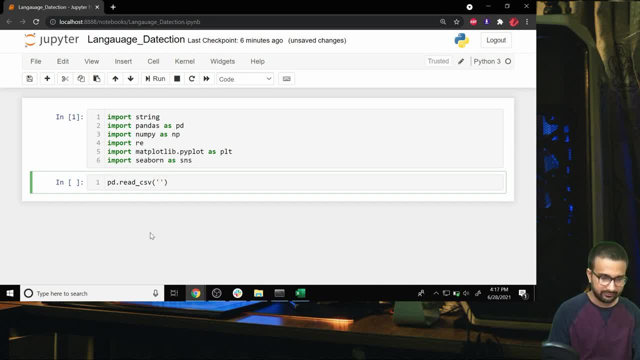 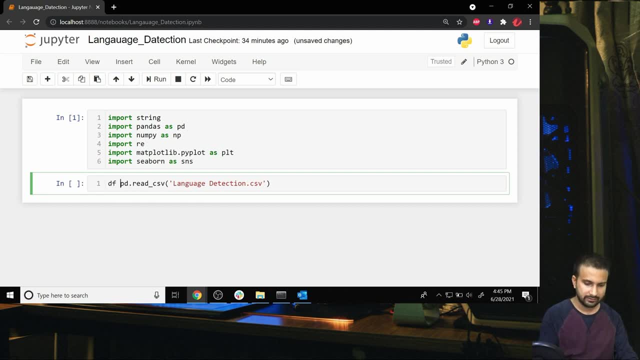 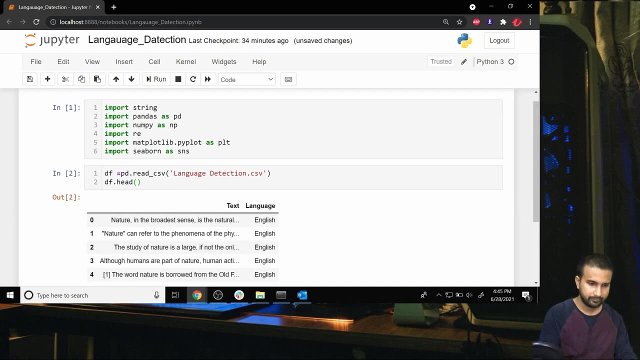 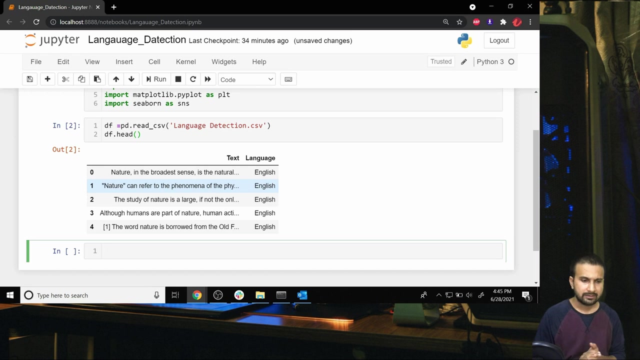 copy path and all, So let's import language detectioncsv. So, guys, let's save this dataset- df is equal to this- and print the head of this dataset. So here is our dataset. as you can see, we have text and languages. 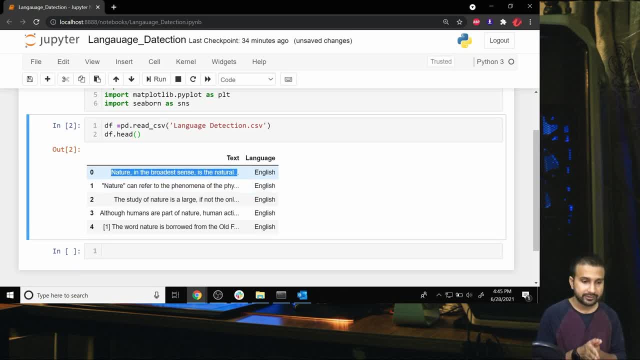 But this data, It's not very clean, As you can see. we have commas, we have double colons, we have dots, we have brackets, a lot of information which is not necessary. I'll say we should clean it out. 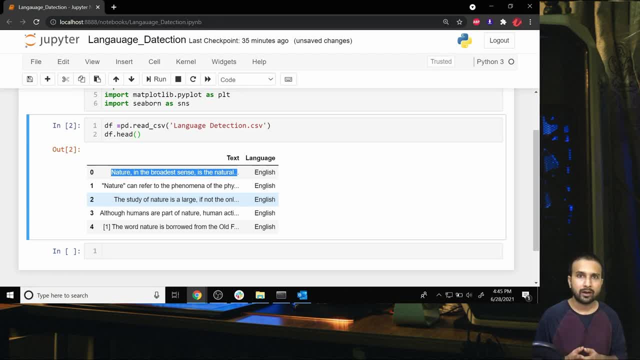 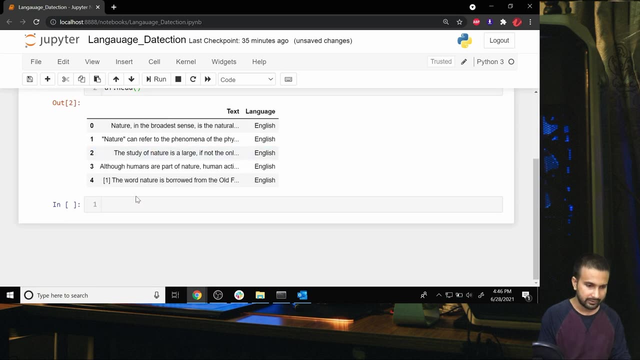 For cleaning up the dataset. either we can write up our own function or we can utilize the Python provided punctuations function, which is a module within the string library. So let's do that, Okay, So if you look out this string library, let me just go down here. if you write P and then 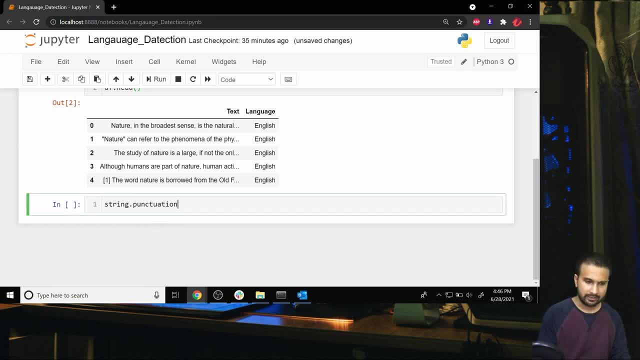 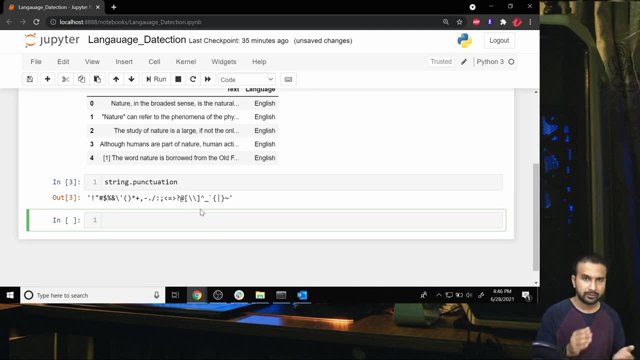 press tab, you will get this punctuations, And let's run this. So this command will give you all type of punctuations. Now you have to remove these punctuations from this text folder. And also, since we have some words which are on the uppercase, some which are on the lowercase, 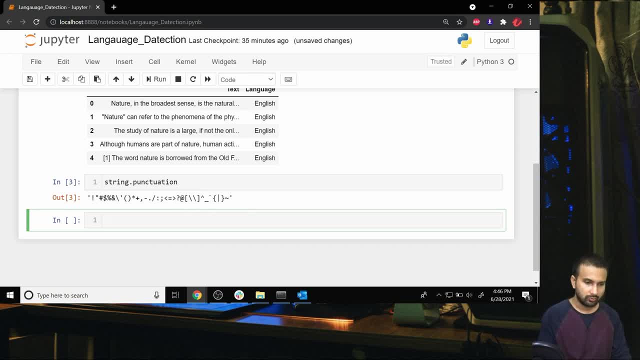 let's make all of them in lowercase. So I'm going to do both the tasks in a simple function, because we need, because, after having a function, we can actually use that function and apply this on top of this data frame. In that way it will save a lot of our time. 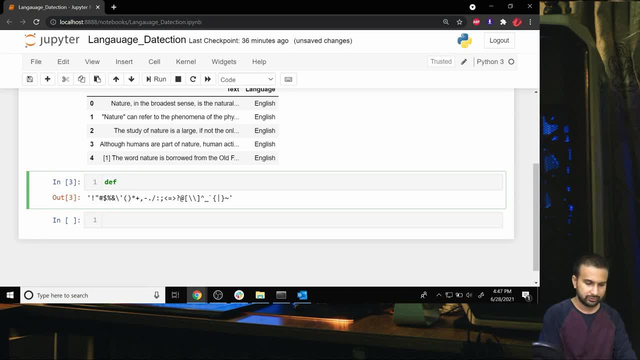 So let's write up a function named H. remove you in now. This takes up Some text, So let's write text. We will write up a for loop and we will iterate to all these punctuation word. So I'll write from string dot punctuations. 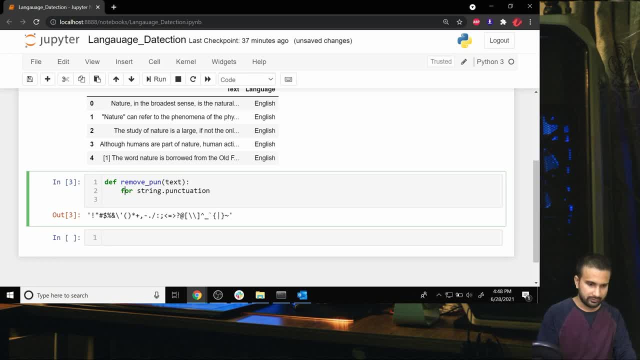 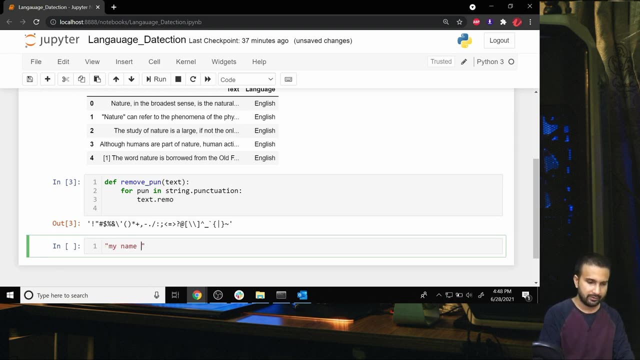 Punctuation, not S, Sorry, So we'll have for pun In this Here. So we'll use the remove command. So if I write my name H J and I want to remove all J out of this line, so I can write replace: 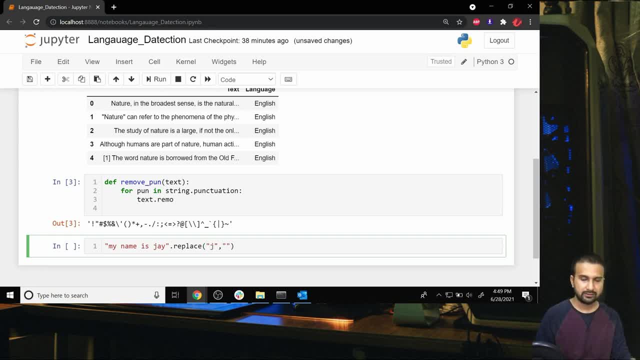 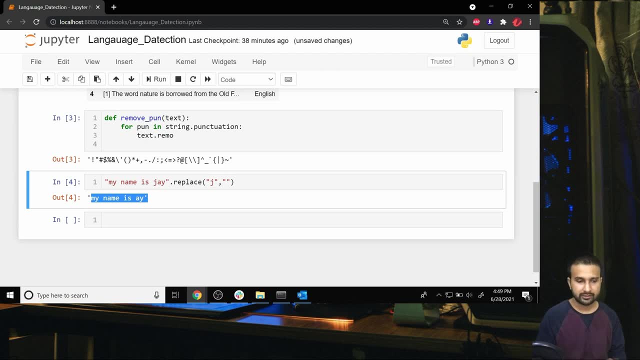 And I can write J over here and then I'm going to replace it with nothing. So let's run this and you can see the J is removed from the string. The same method will apply on this text. So let's run this and you can see the J is removed from the string. 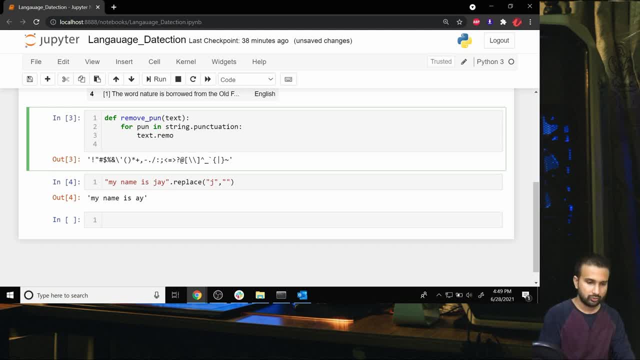 The same method will apply on this text. And since it is iterating on, this pun is actually iterating. And since it is iterating on this pun is actually iterating, So he'll write pun to this double colon. Then we also need to save it. 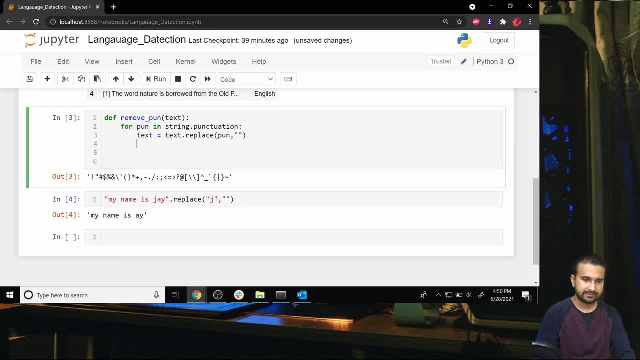 So we'll save it inside text only. So like text equal to text, dot placed pun double colon. Now we also want to make that. Well, let's say in this we have a word dot function lower case, so after the removal I can write: text is equal to text dot lower. so 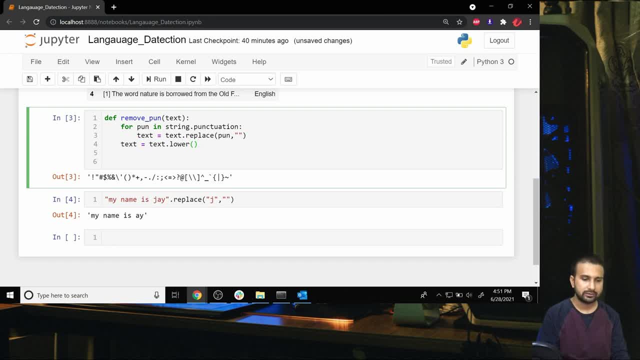 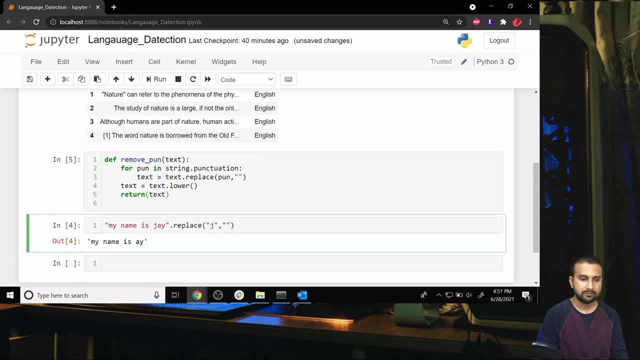 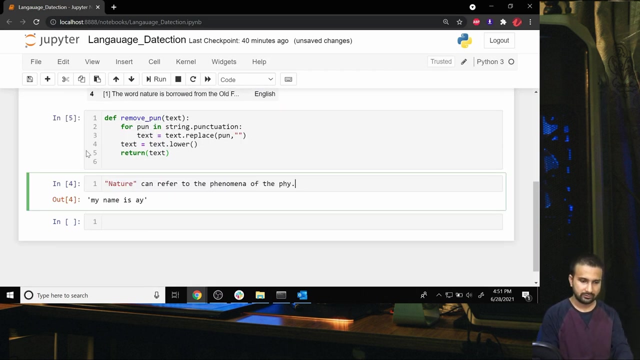 it is going to completely lower down the caps, or the uppercase letters, and this we are going to return now. okay, txt. now this is our function. now let's apply this function on top of some strings which is coming over here. so, as you can see, nature can refer something like something. so I'm going to write down. 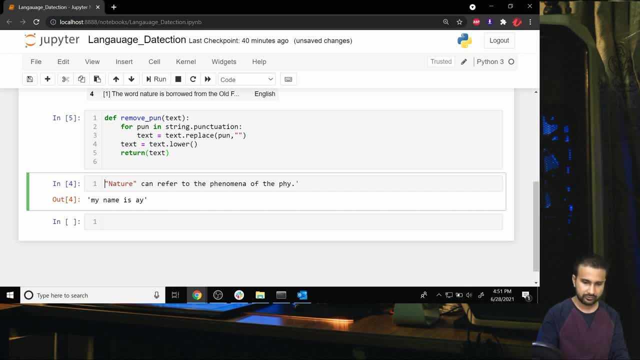 this over here and let's do this now. I'm going to pass this complete string to this function and look that this function is working correctly or not. let's put some other punctuation also. I like double colon, and then this: and now we build up, apply this function, remove UN, Wow. so, as you can see, all this. 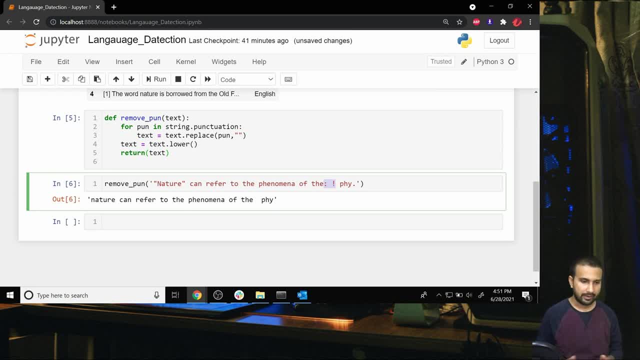 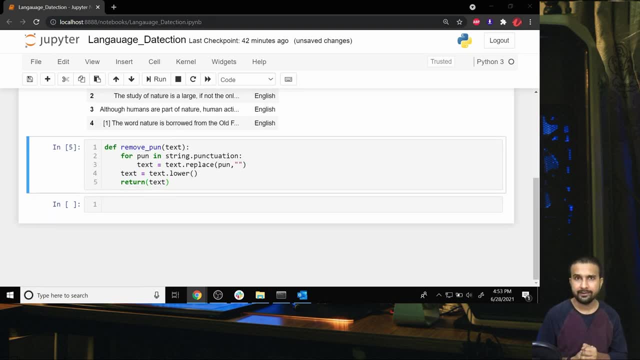 x- military mark, double colon. everything is gone and this function is working pretty well now. the benefit of having a function on hand is that I can actually apply this complete function on top of this data frame. so let's apply it and see it's working fine or not. so we can write DF dot or we can write VDF text. write down this function. 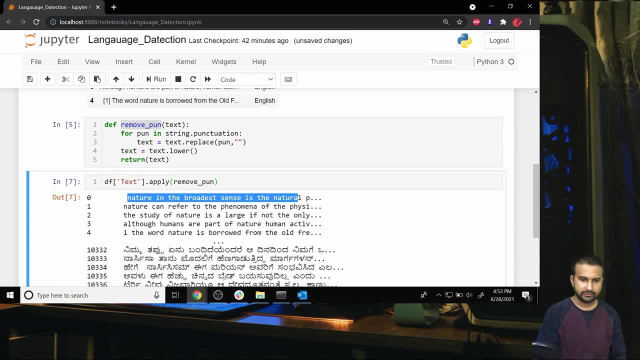 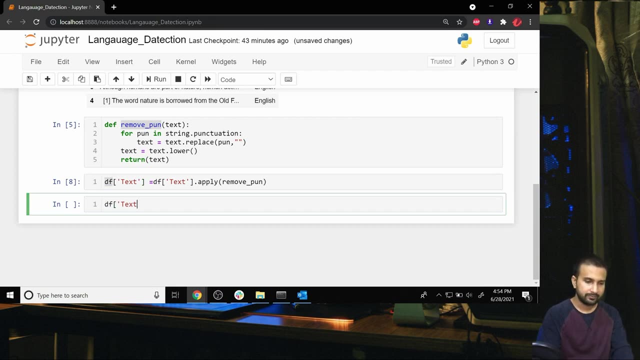 name and let's see so. as you can see, everything is working fine. we are being able to apply this function. now let's save this- new values and here is our data frame with somewhat clean data frame- and let's save this function so that we can data. 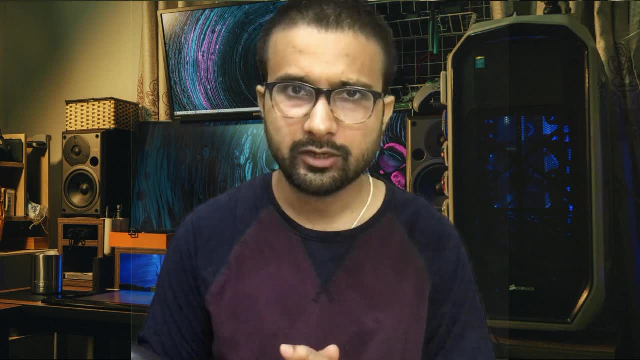 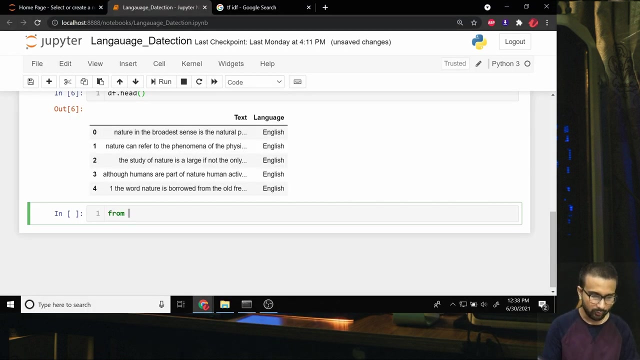 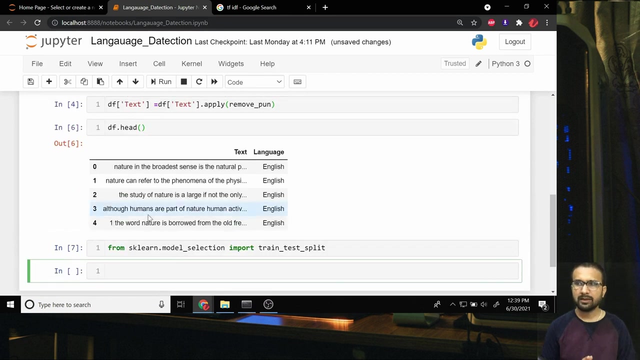 So, guys, we have done some basic cleaning on top of our data set. This is the time to divide our data set into training and testing splits. We will be using the train test split provided by sklearn library to do the split over here. So let's import the train test split from sklearn, but before we apply the train, 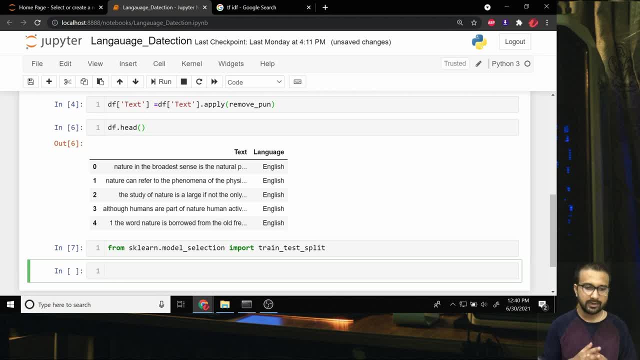 test split on top of this data frame. we actually need to have our X and Y as in separate values, So we will use the ilog command. So, since our text, which is the X values, this is in the 0th column, so we'll take all rows and 0th column over. 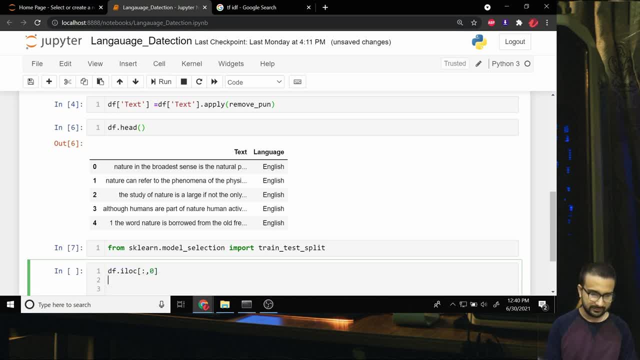 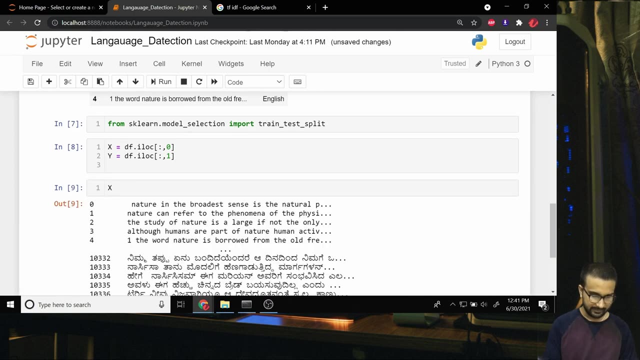 here and in the Y's we will take all rows and the first column. Let's save this within X and this within Y. Let me print this X also. So, as you can see, here we have all the X coming out as in single series and you have Y also, which is having all the 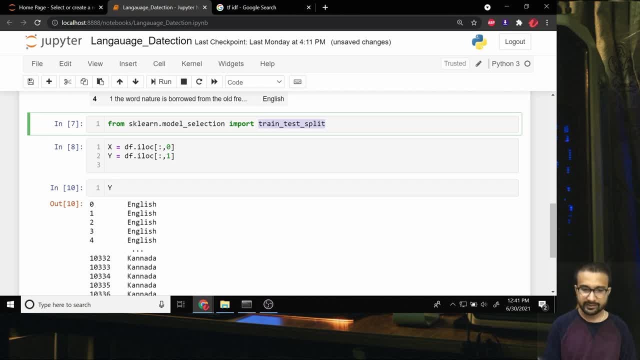 languages. So this is good. Now we will apply this train test split function on top of this- X and Y. So we have to give X over here, We have to give Y over here. Then we can give how much percentage of the total data set we want to keep in. 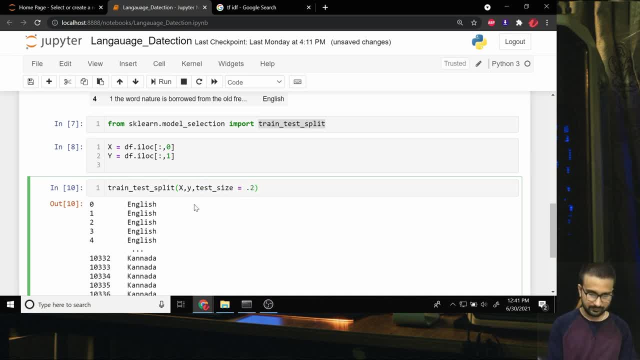 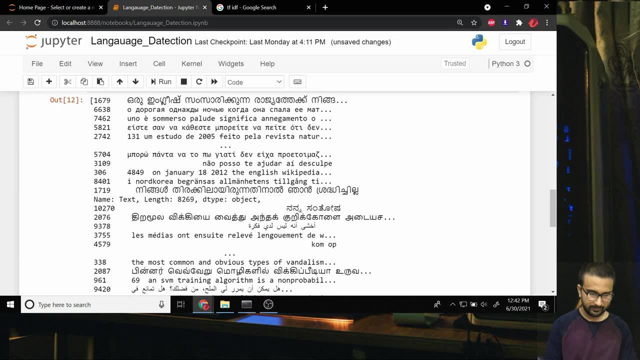 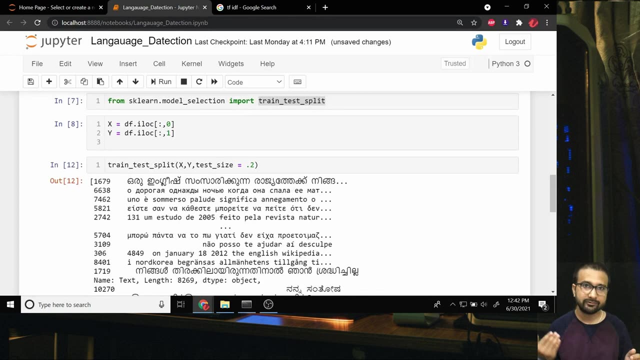 the testing side, and here you can give around 0.2.. So this should be caps Y. This actually returns you four values. The first one will be X train, then what. the second one will be X test, then Y test, train, then y test. so let's save this within variables: comma y train, comma y test. 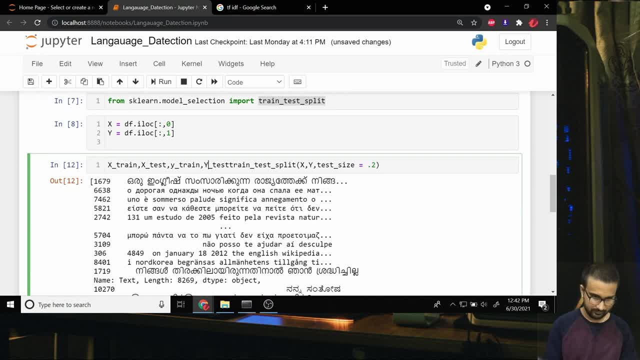 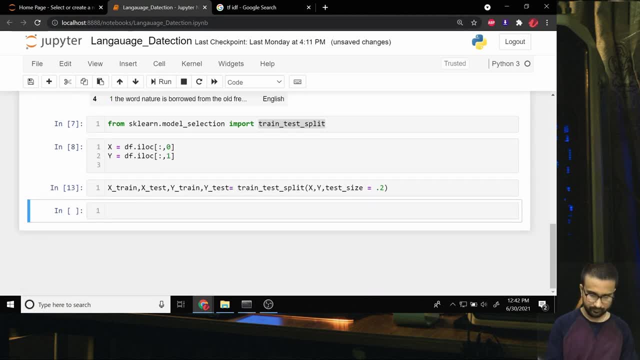 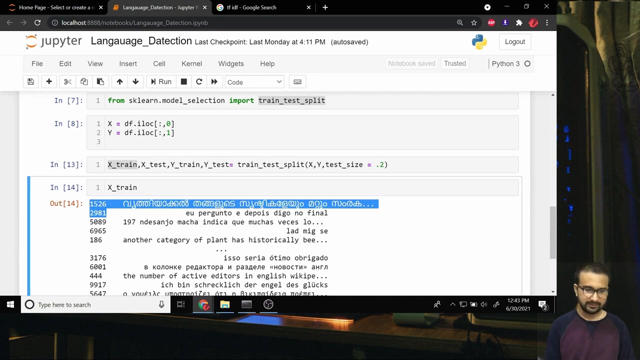 i should have this also in caps. now these are four values of x, y and actually i can print them and we will just clarify that our values are coming correctly or not. so you can see we have x and here on the index side you can see the first index is 1526, so it means the values are randomly selected. so this function is very 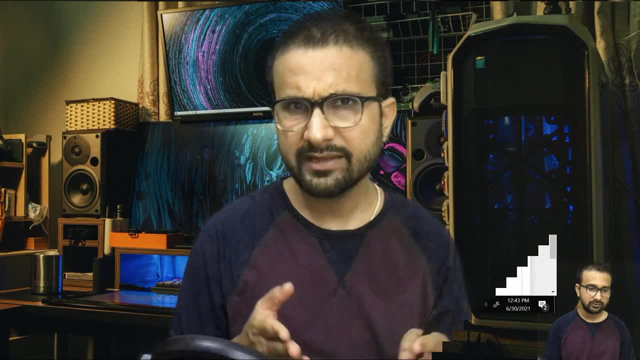 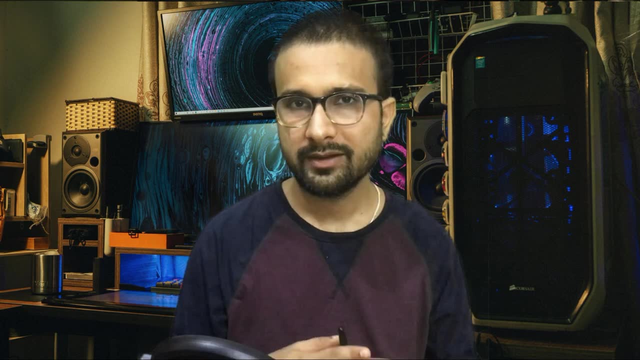 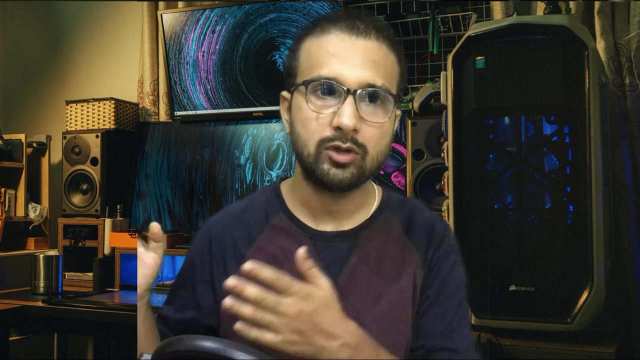 good, you can use it in any type of algo. you can use it in any type of algo. so, guys, we have splitted our data set into training and testing part, but there is something missing over here. our model cannot absorb these string values. i cannot feed this complete sentence to our model and tell and ask model to do some calculation on. 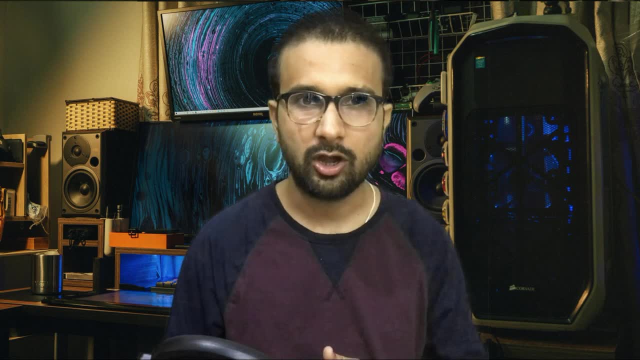 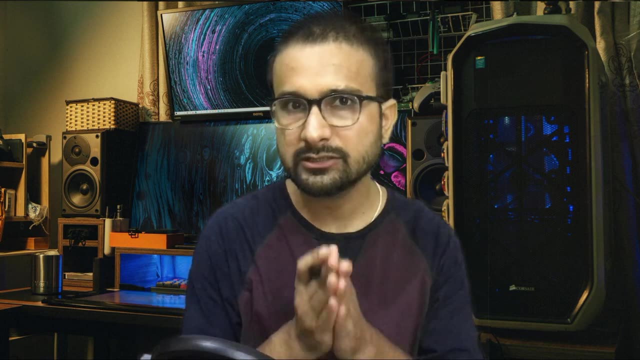 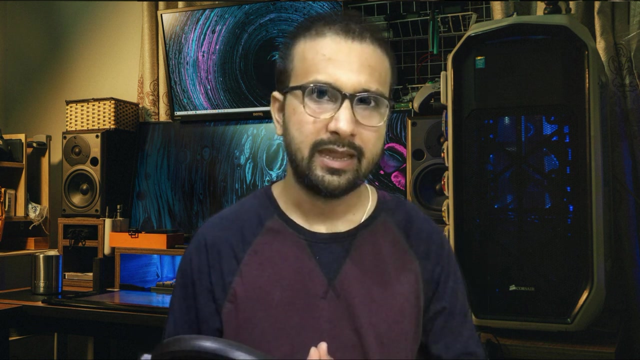 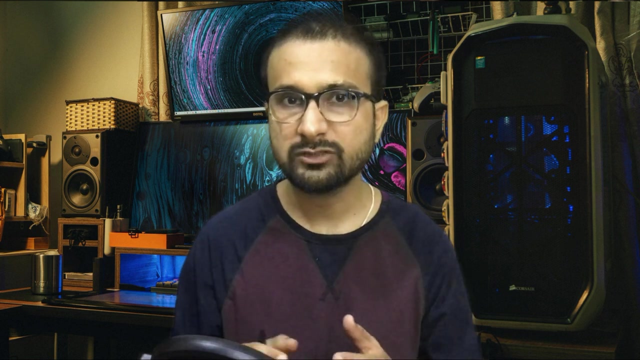 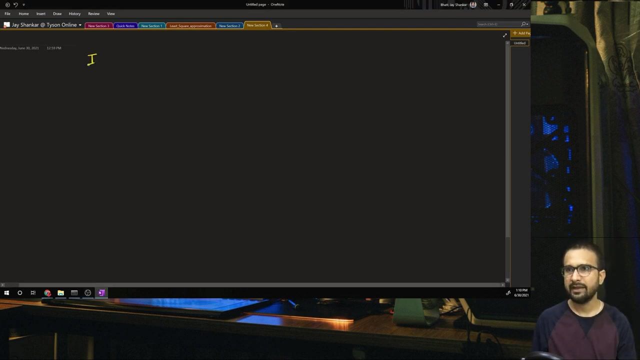 top of this. so there comes the use of vectorization or converting these strings into some feature or numerical value which my model can understand. ok, i have understood. you flushed out what you had just understood and there are n number of ways to do so. i'm going to talk about uni-gram, bi-grams and tf-idf technique over here, before we get into the actual coding. 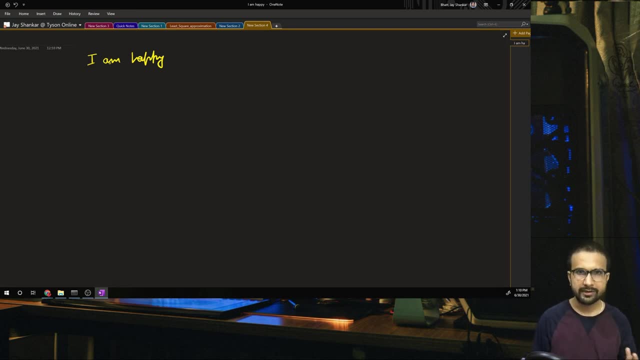 let's understand how the techniques actually works on the background. so let's understand this. with an this. I am happy to a vector. what can I do? So the best thing I can do that I can just figure out how many unique words are appearing within the sentence, So I 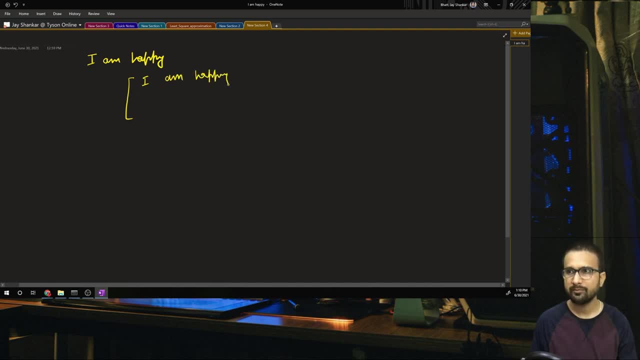 have I, I have M, I have happy. Then I can give these, as in unique features, like I am happy. So I will have one feature named as I, the other one is M, the third one is happy And I can count how many times they are appearing. But in case of 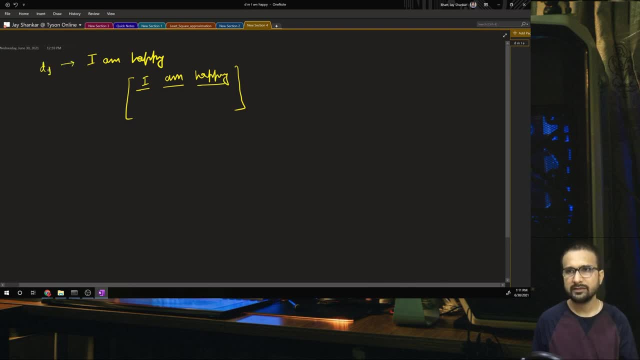 NLP. we usually say them as in document, So we can say small t1. And in that way you will have other sentences also like document 2, which is saying I am unhappy If I have these two sentences. I can see that I and M are unique for both the 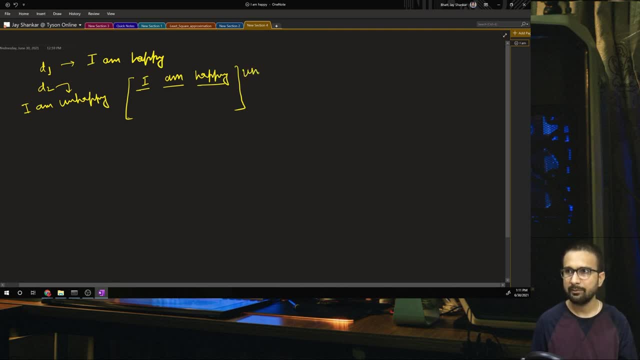 sentences. The next thing that I can take is unhappy. Now I have four features in my vector And I can actually count how many times these features are appearing within my documents. Like for d1, I is appearing one time, M is appearing one time and happy is appearing one time, But unhappy is not. 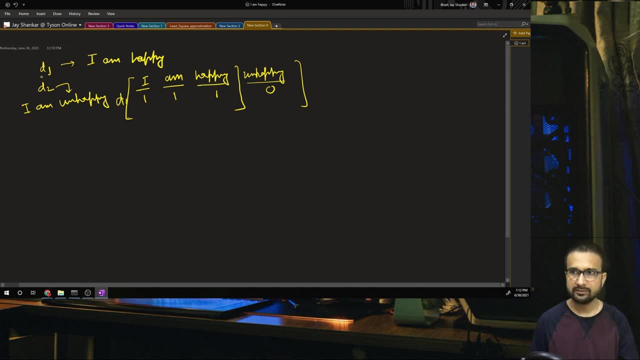 there, so we'll write zero. So this is a vector and this is for d1, the first sentence or document. Now, if for d2, I have I, I am happy, But happy is not there, so I will write zero and then we have unhappy. Okay, simple. 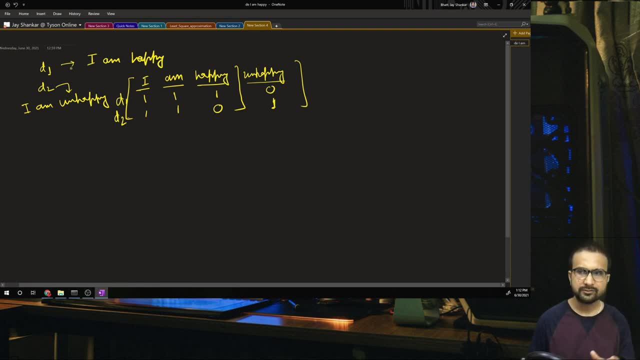 So right now we are taking individual words into consideration. So if I say this sentence, I am happy, and if I say, am I happy? Now, these both sentences are completely different. but what is happening over here? I'm getting two the same sort of vector out for both the sentences. 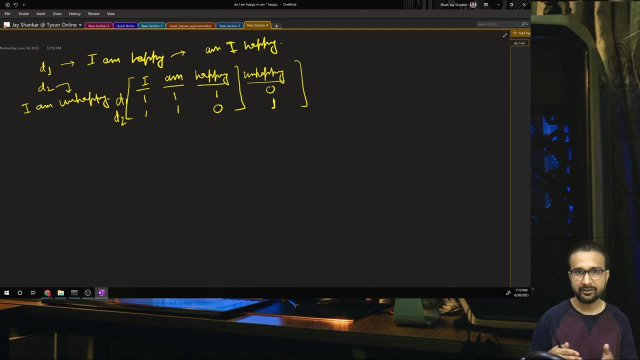 So in some way we are losing some sense of continuity over here or the relation between two words. So this technique where we take only one word, is called unigram. If you want to consider the connection between the words, we can go into bigrams. 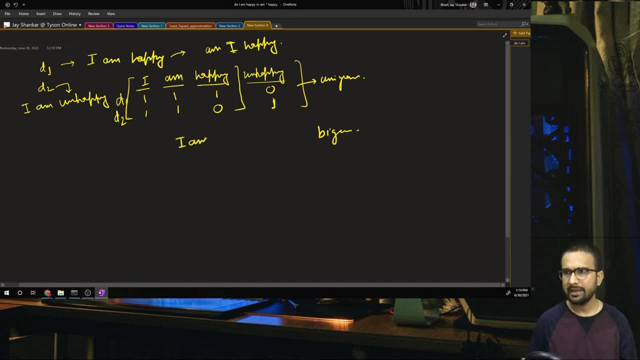 Now, what is bigram? In bigram we take, I am, as in one feature, then am happy. as in second feature. In the second one you will have, am unhappy. So you are taking two words into consideration. That's why it is called bigram. 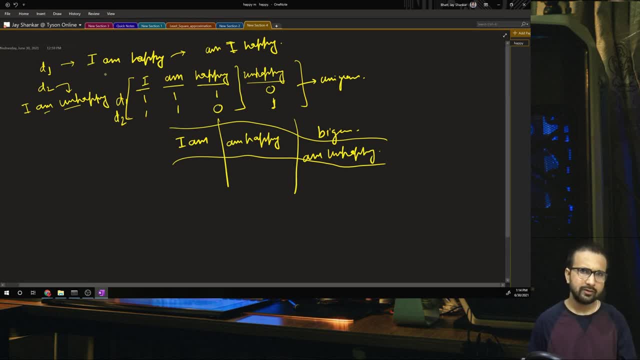 Now, if you see you can go even for trigrams. There you are taking three words in continuity as in single feature, So I am happy itself becomes a feature out there. This is the story behind unigram, bigram and trigrams. 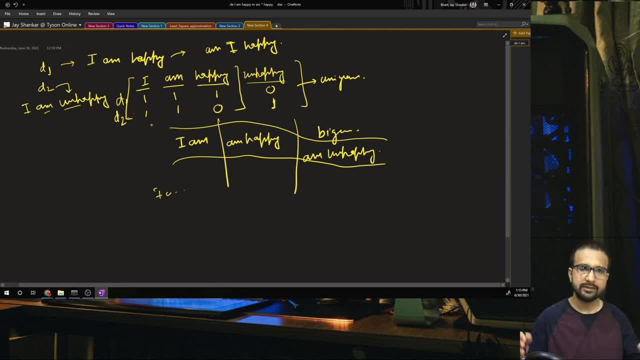 In the case of model training, you can actually take all three into consideration, where you are having your unigrams as well as your bigrams, as well as your trigrams. So these all will become features for one document And in this way, you can have multiple documents, as we have a big data frame. 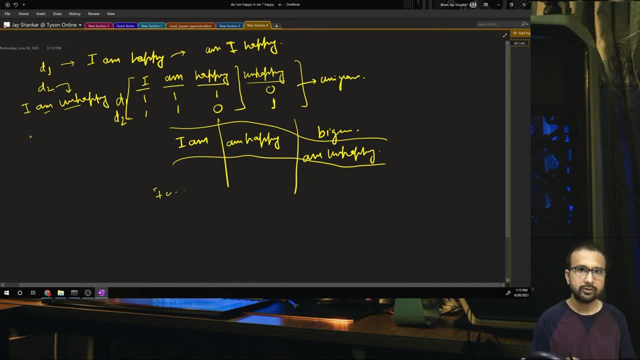 All the sentences are called individual document. You figure out the unique words out there, Then you create up this sort of vector form where you have how many times the word is appearing within the sentence. This guys have some issues. again. There will be many words in a language which are very, very frequent. 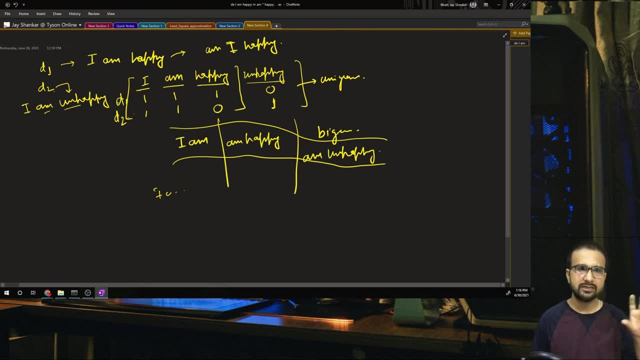 Like we say in these two sentences: if I want to see there is some difference between the two sentences, unhappy and happy words are giving the most sense out over here. If I see the I am words over here, they're not making any difference between the two. 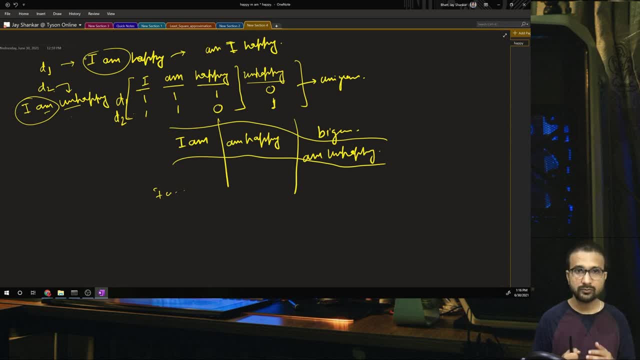 sentences. But happy and unhappy are the words which are making a lot of difference over here. So why not give higher weightage to happy and unhappy And give lower weightage for I am? So there comes the TF IDF technique. So TF is the term: frequency within a single sentence or a document. 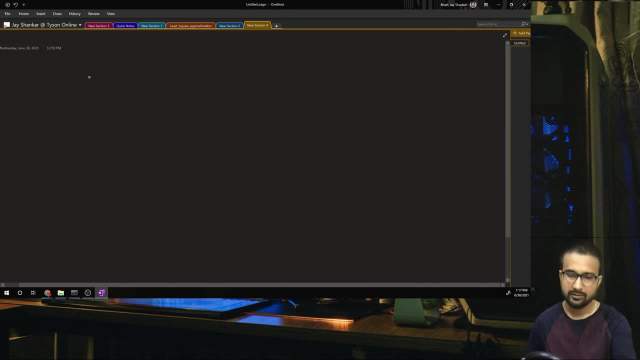 Let me clean this out so that we can do it. We have the sentence now I am happy, And other one, I am unhappy. Now, in these two sentences, let me write this as document one and document two, If I see. so what will be the term frequency over here? 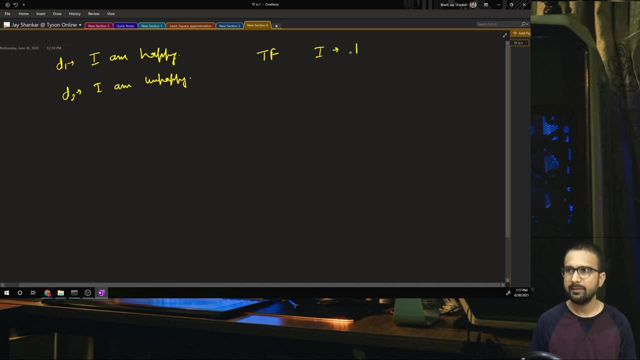 So term frequency for D1, if I see for I it will be one divided by the total number of words. So I have three words, so it will be one by three. For M it will be same: One by three. 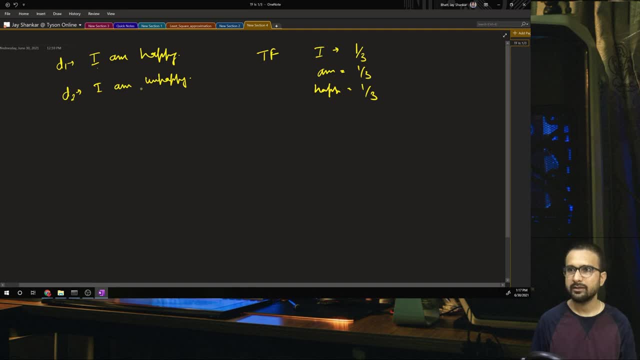 For happy. it will be same: one by three, And that goes with the D2.. You will have so why I am doing divide by three. I want to take into a calculation sort of which is ranging between zero to one. That's why I'm just dividing it. the total number of words within document. 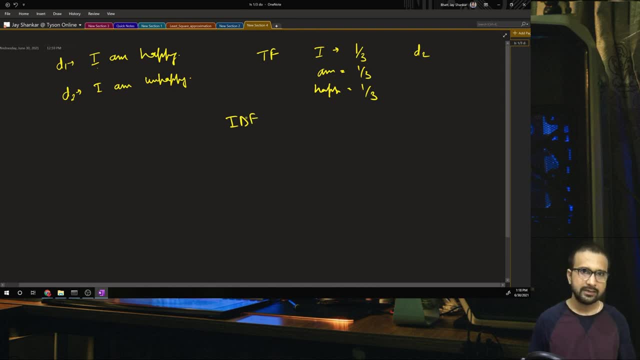 Now, what is IDF? So IDF is the inverse document: frequency. So if I see so, the IDF- for I will be how many times I is appearing, both of the sentences, So the total number of sentences or documents will come into the denominator, and how many. 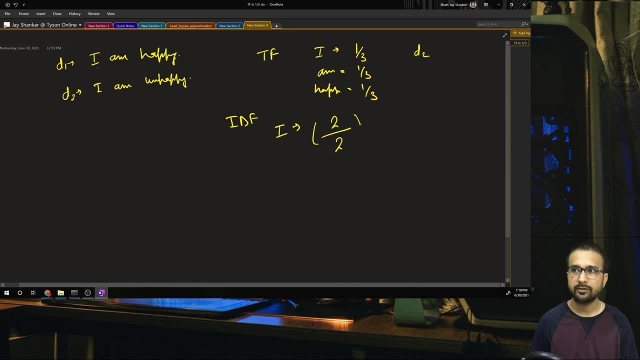 times I is appearing over there will come into the denominator And you just have to take the log of this value. Okay, So log of one will be zero. Now, if you multiply This TF and IDF of this I, I will have one by three multiplied by zero, which will make 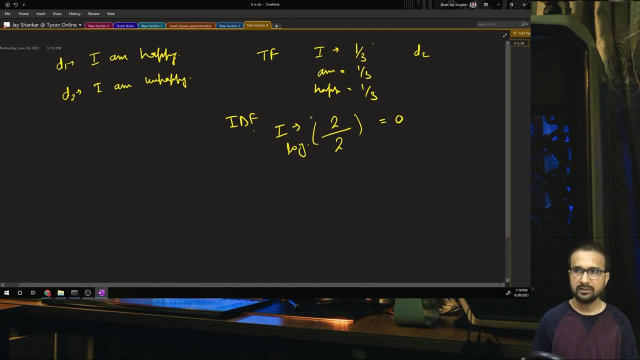 this complete TF multiplied by IDF. zero for this. But in case of unhappy I will have, since we have two documents. so I will have two in the denominator but I will have one in the nominator because it is only appearing in the first sentence. 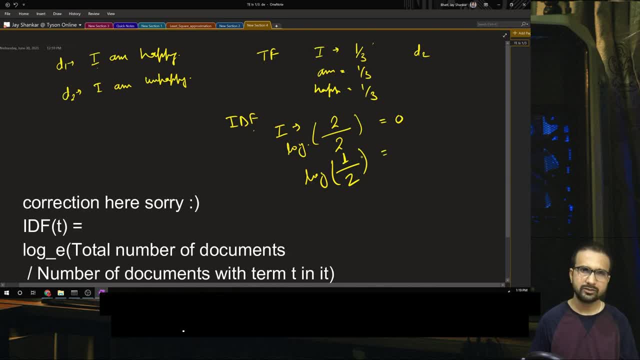 So the total value will be log of 0.5.. That will give you some value. Once you apply this to this value, once you multiply this to this happy value over here, you will get some value out over here which will not be zero. 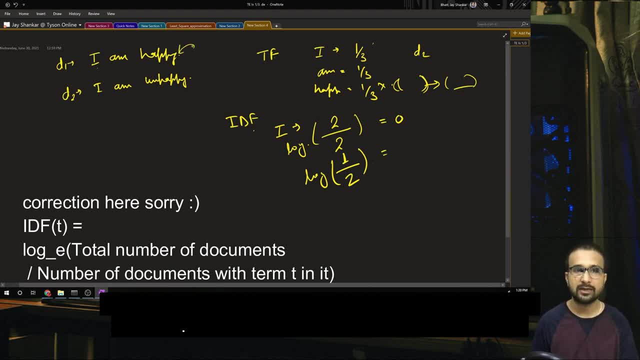 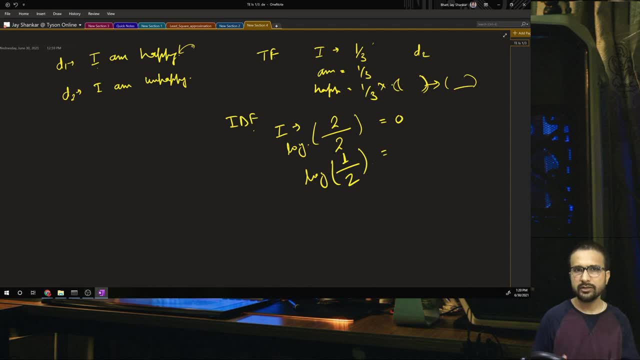 So in this case, you are giving the higher weightage for the words which are appearing least in the document and having the higher impact. So this is the concept behind the unigrams, bigrams, trigrams and the TF IDF. Now we will write up the code to figure out or create a vector. 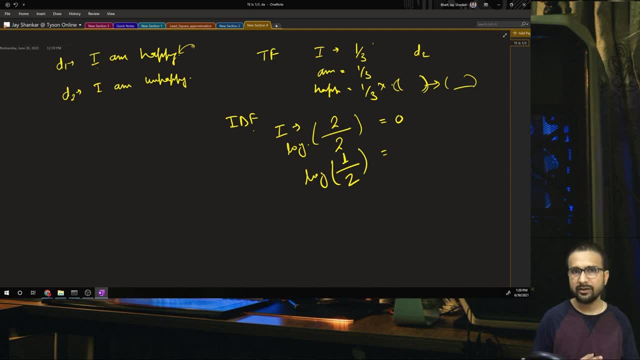 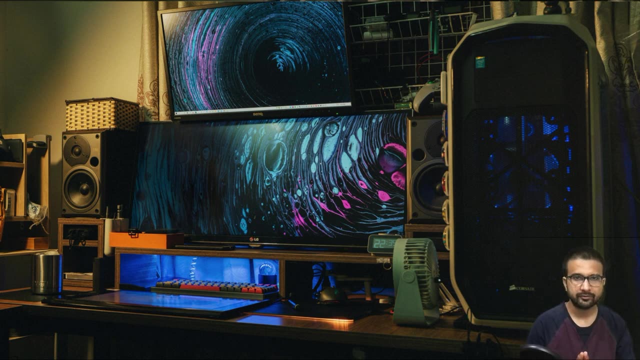 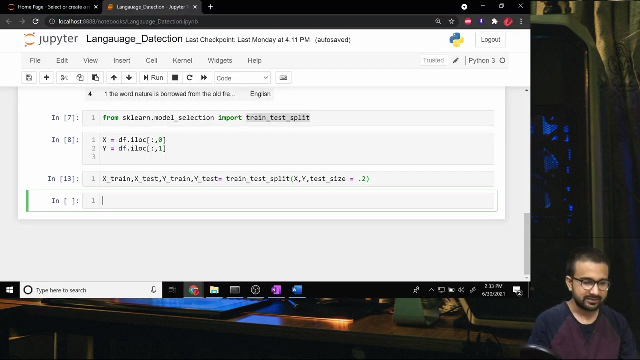 Okay, Now create a vector matrix out for our document, feed it to a model to train up on top of them. So now we understood the theory behind TF IDF. Now let's vectorize this data set and create the features. So as long as it sounds in the theory side, it's very simple to code it out because we 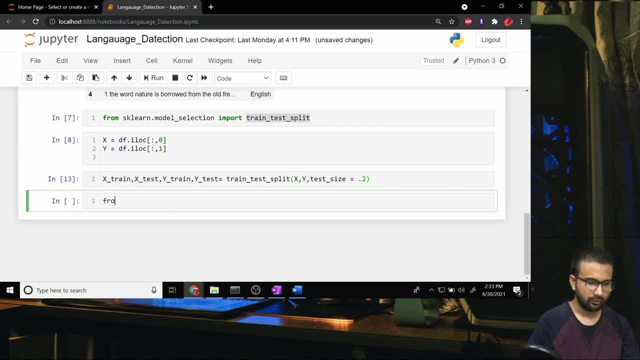 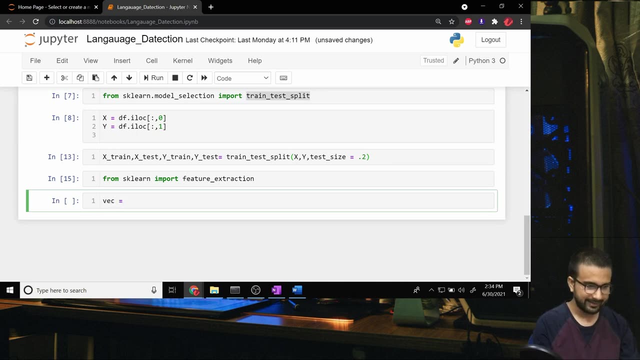 have a library available from sklearn, From sklearn import feature extraction. Now with this library, if we can actually create a vectorizer, I'll say vec is equal to feature extraction, dot, text, dot. So we have TF, IDF transformer vectorizer, So we have to use the vectorizer over here. 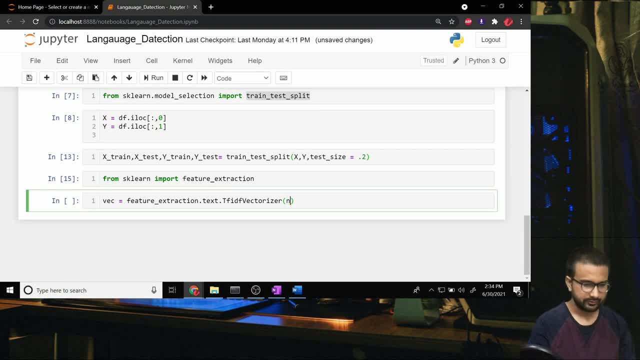 So over here you have to give the engram range. So, engram range, as I told earlier, we have, Okay, Okay, Unigram, bigram tigrams. So we are giving. if I give one comma one over here, it is going to take the unigrams. 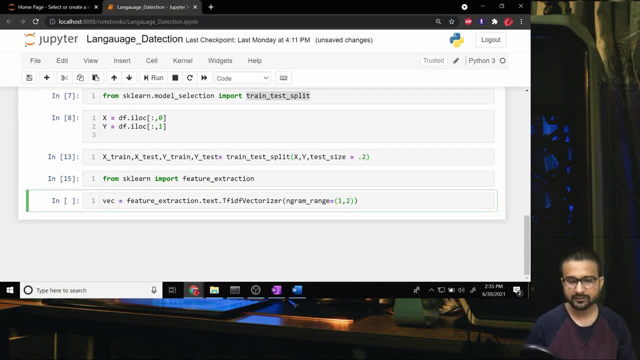 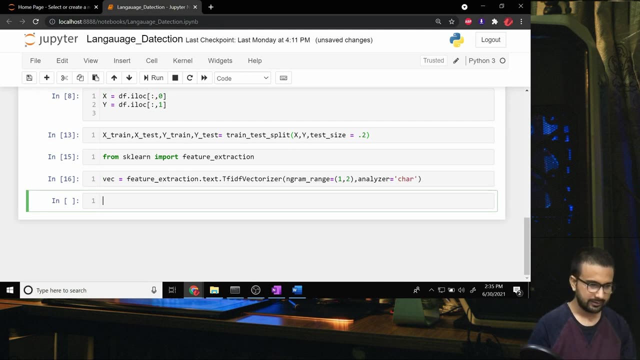 If I'm going to give one comma two, then it will take unigrams and bigrams. So for now let's take one comma two, and here we have to give the analyzer, That will be char, As like other sklearn models, We cannot directly go ahead and train up our model here. 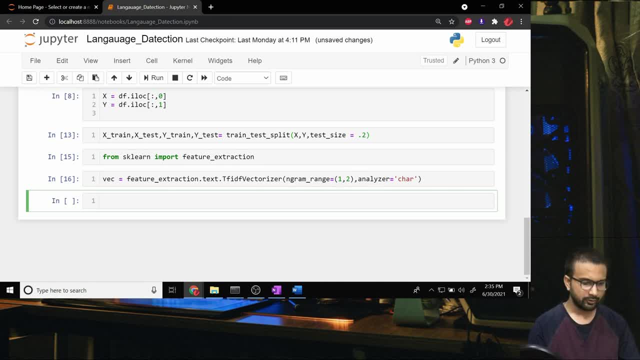 So we will be using something called as pipeline. So I'm going to import this pipeline from sklearn and then we are going to define this pipeline. So pipeline is something like if you want to do some sort of continuous work, where you are first converting your text to a vector and then also training it out, you can create. 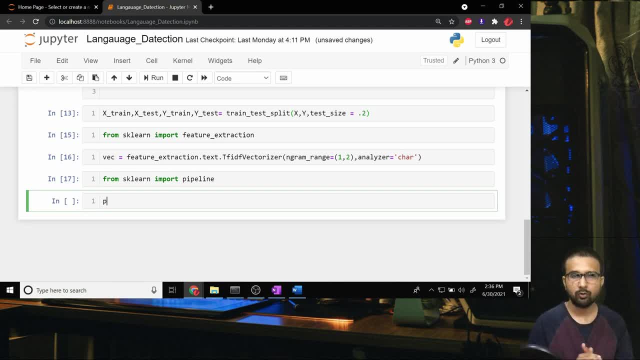 up pipelines, So it's kind of creating up a complete flow, Okay, Of functions. So for doing the pipeline thing we have to just write pipeline, dot pipeline, And inside bracket we have to define what all tasks we want to do. 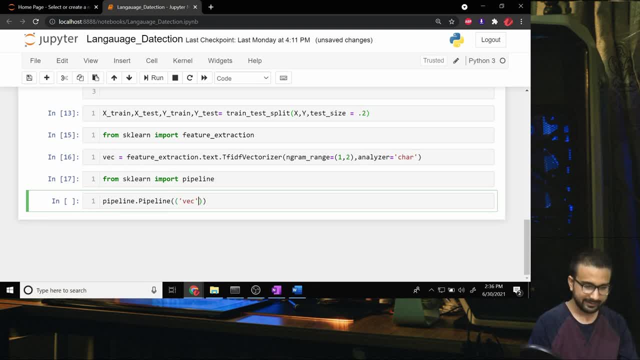 We want to apply the vectorizer, So I'm going to write vac comma vectorizer. This is the same vectorizer that we have defined over here. Once this terms gets vectorized, we want to apply a model on top of this. For now, I'm using the logistic regression. 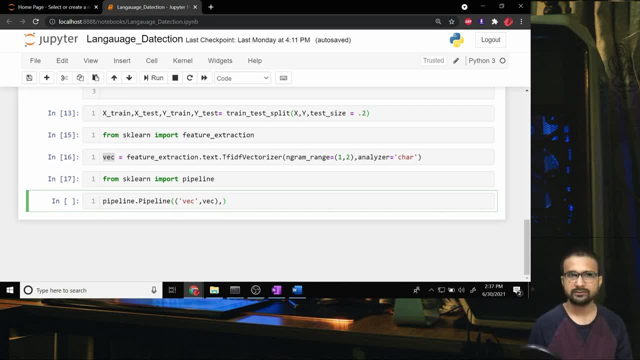 You can apply other models like lgboost, random forest or simple decision trees, whatever you want. So we have to give a name for that pipeline component. So I'm going to write CLF. We have to import the model first. So I'm going to use this linear model from sklearn which have logistic regression model. 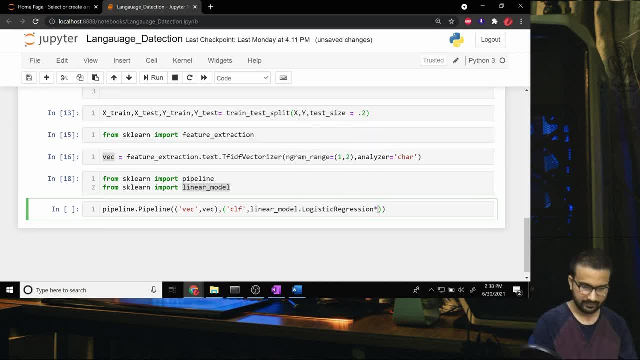 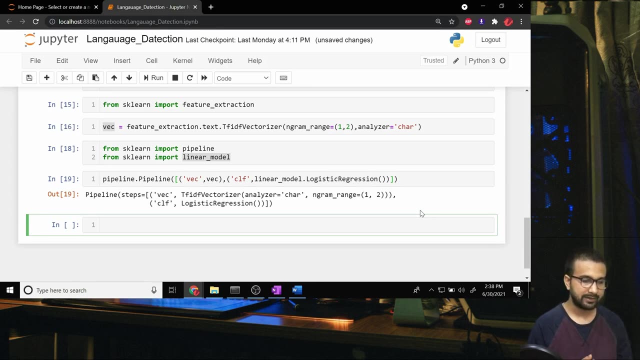 You can just select this logistic regression bracket. This all pipeline components you have to write within a square bracket. So this is something like a list form you need to write. So once you will run this, you will see that it has created up a pipeline which have multiple. 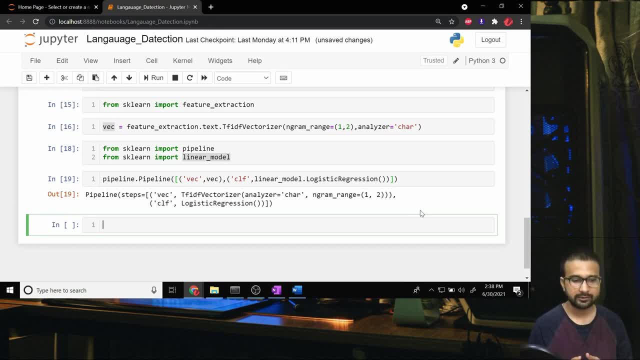 steps. In the first step, it is going to take up your string, convert it into a vector form. Then it is going to train up the model Once you have defined your pipeline. it's very simple to train up your model now. 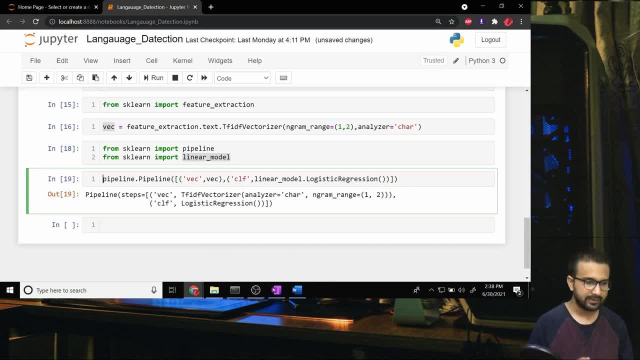 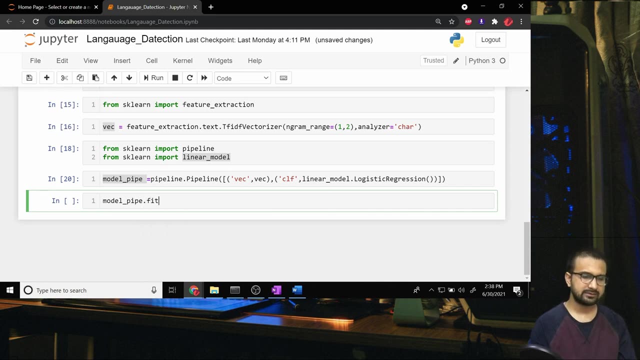 So let's save this pipeline component within a variable. I'll say model pi, P-I-P-E model pipe- Oh, I should have had some better name, but who cares? So dot fit. So it is the same way how we actually fit up the model for other sklearn methods. 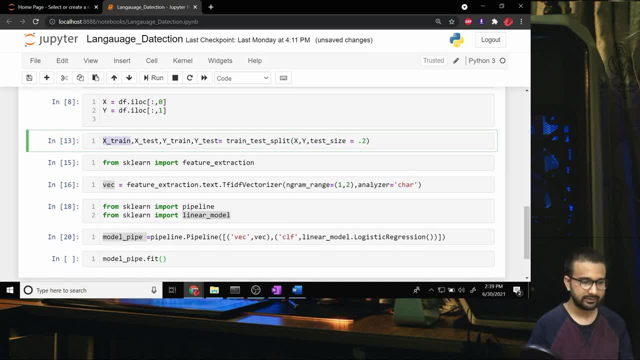 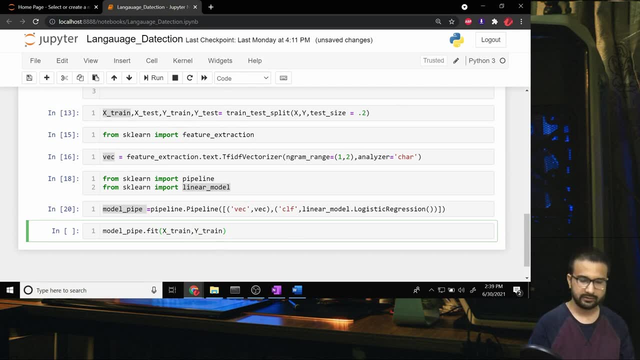 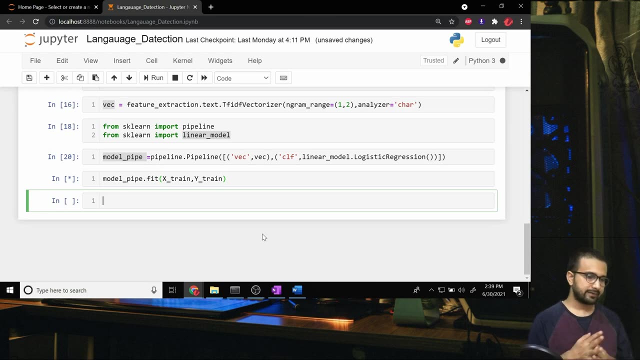 So here you need to give the train component. So I'm going to give the x train and y train And let's run this, Okay. So once you will run this now on the background it is converting the complete data set into vector form and training up your model. 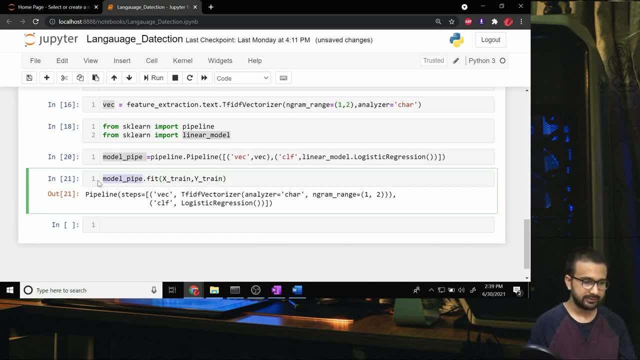 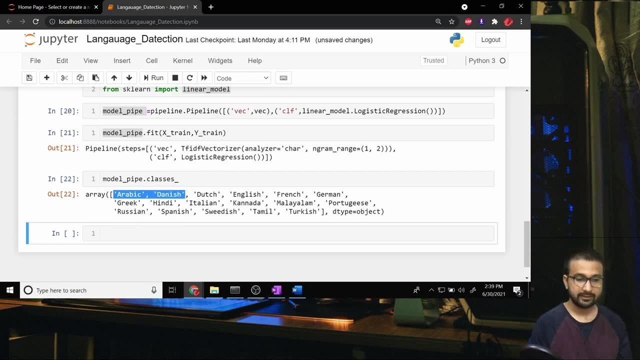 So this is all now. our model is trained and you can actually see your model components over here. So you can see like classes. So you have these, only these many languages over in that y variable, like Arabic, Danish, Dutch, English, French. 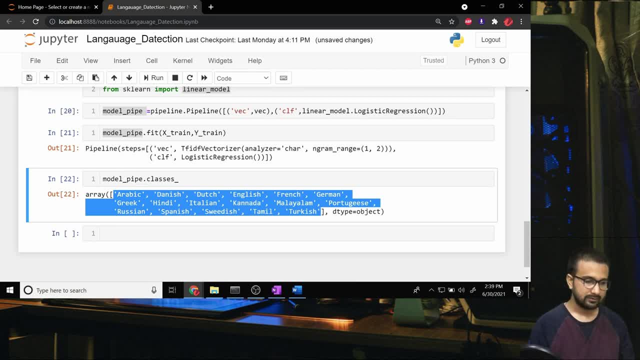 All these languages are there in that, in that data set. Now let's try to analyze this model and see how accurate it performs. on the testing data set, We will apply the predict method and we'll give the x test over here. So this is going to predict the y values for all the words which are in the testing data. 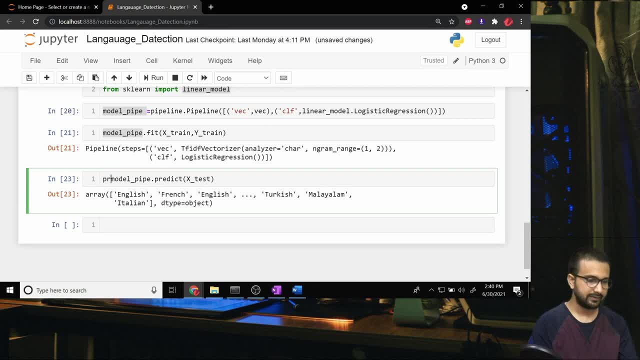 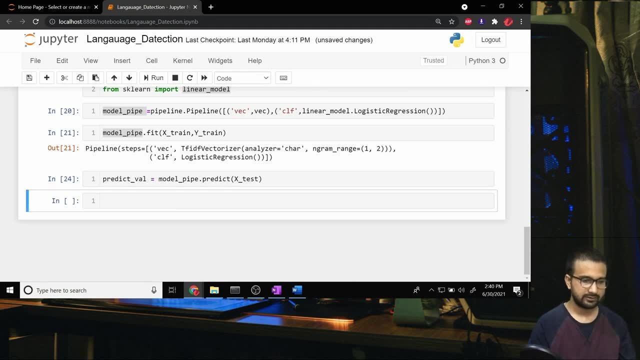 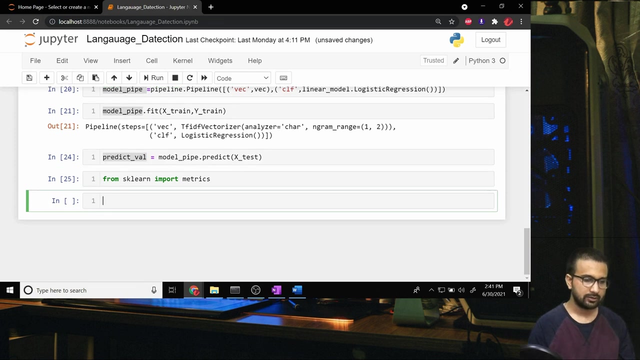 set, And here is the predicted one, So I'll save it within a predicted variable: Predict. Well, Okay, So this is our variable, which contains the predicted levels. Now this is the time let's calculate the accuracy. So, sklearn, have this matrices which can actually give you the accuracy of the predictions. 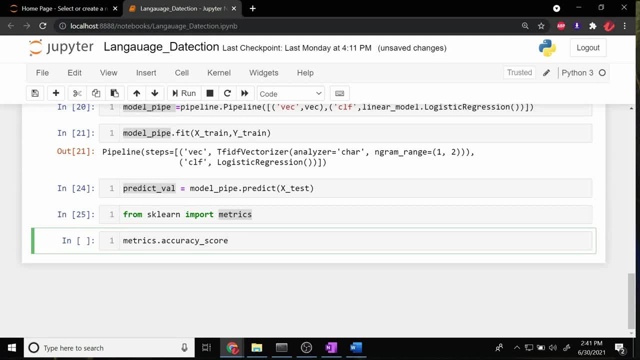 So within the matrices you can actually apply this accuracy score And this one you can give the actuals versus predicted. So I will just check it takes y true and y predicted. So I will just check it takes y true and y predicted. 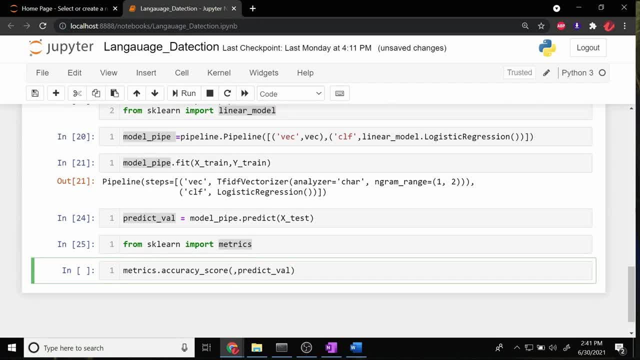 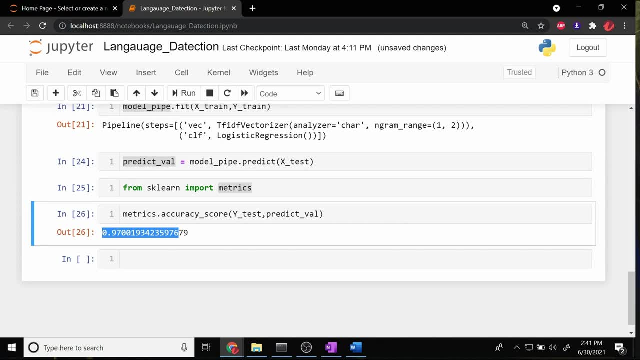 So These are the predicted values and you have your y test. These are the actual values. So here it comes: We got 97% accuracy. Let's apply, Let's multiply this by 100.. Yep, So we have this 97% accuracy coming out with this trained model. 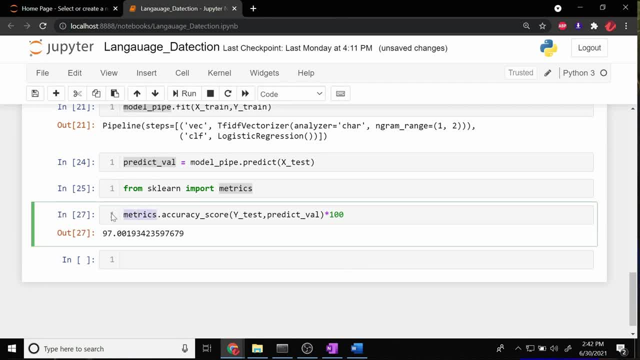 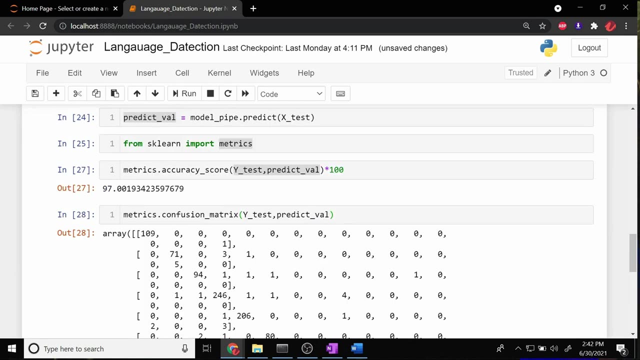 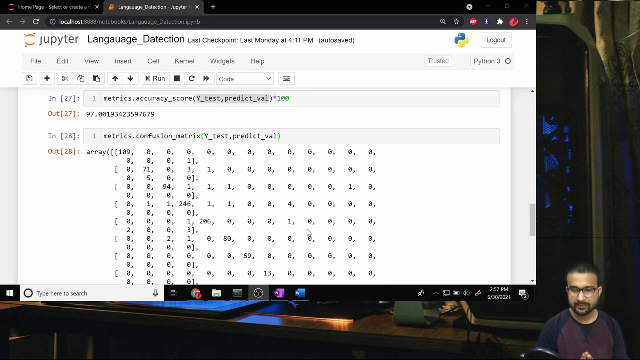 Now you can actually see how the confusion matrix looks like. So, within the matrices itself, You have confusion matrix Which actually takes up the same arguments, and here it comes. So, guys, here you can see the confusion matrix is coming pretty well. You can use Seaborn to create a better visualization. 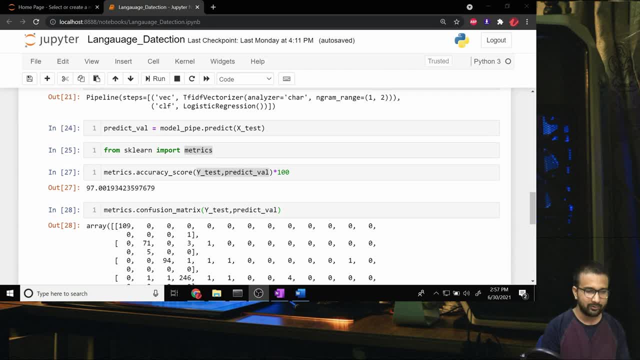 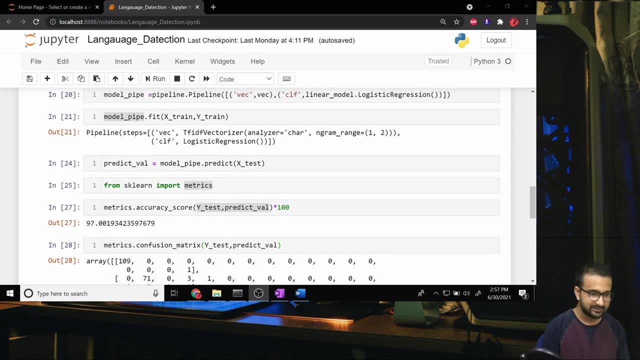 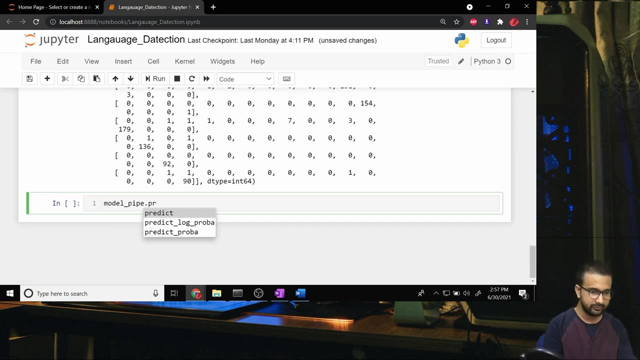 But now my focus is not that. I want to test my model for multiple languages by giving a string on time, So let's do that. So I will take this model, pipe over here, Okay. Okay, This one, And let's go to the next cell and we'll use the predict method and let's give some words. 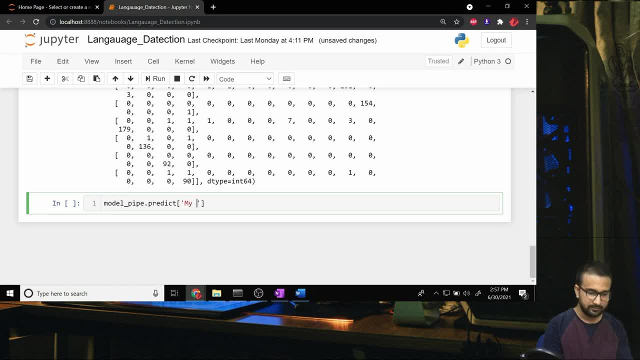 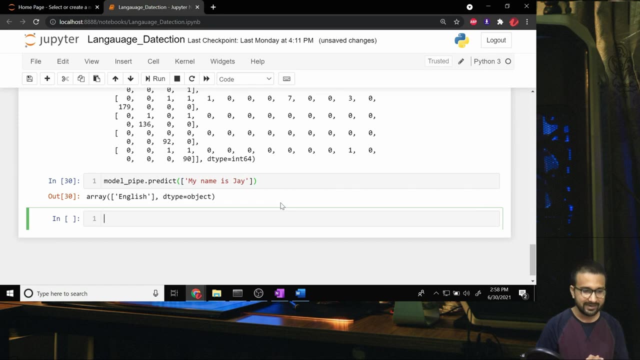 in English. So I'm saying: ah, my name H J. Okay, Let's run this. Okay, I think I have to put up a bracket Now. let's run this And you can see it's predicting pretty well. 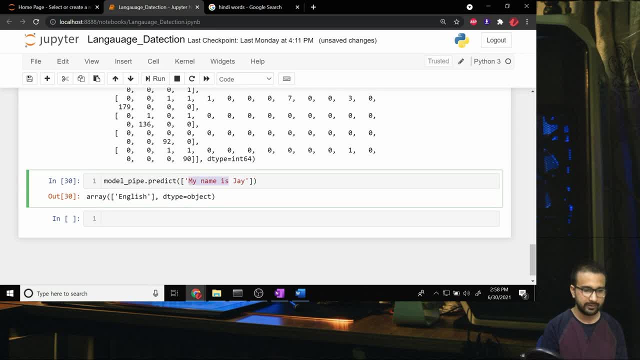 The English word is coming pretty well over here And put it over here. Okay, Now it should give the Hindi word on top of it should give the Hindi language. Let's see Awesome, So you can see it's, it is able to detect the language pretty well. 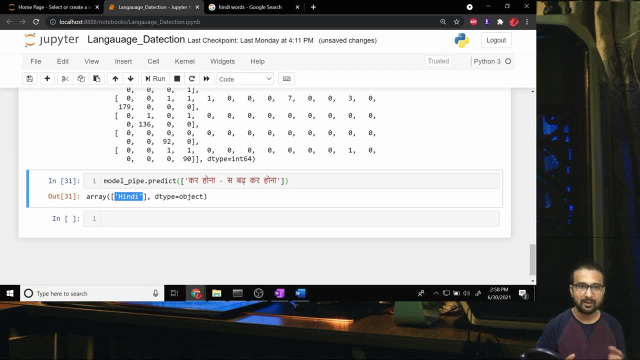 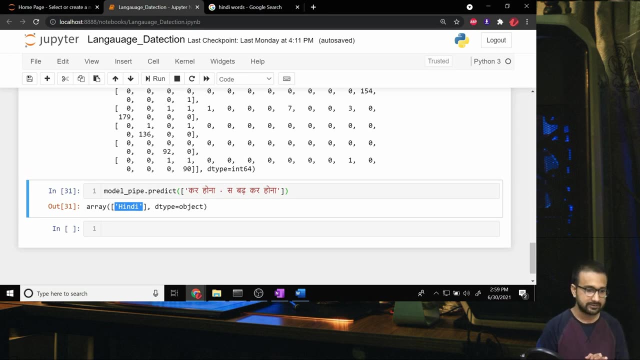 So, guys, again, before we go ahead and create the web app out of this application, please, please, please, please, subscribe this channel, because that gives me a lot of support to create such videos for you guys. Okay, We are good. 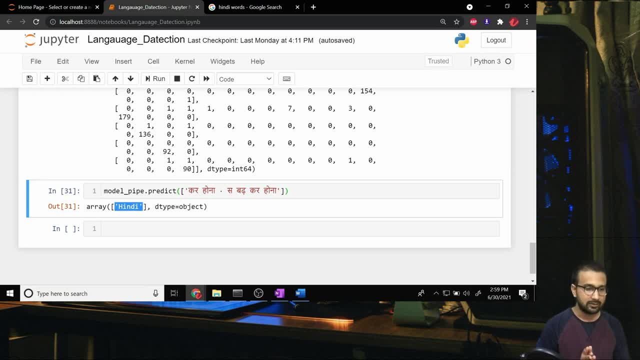 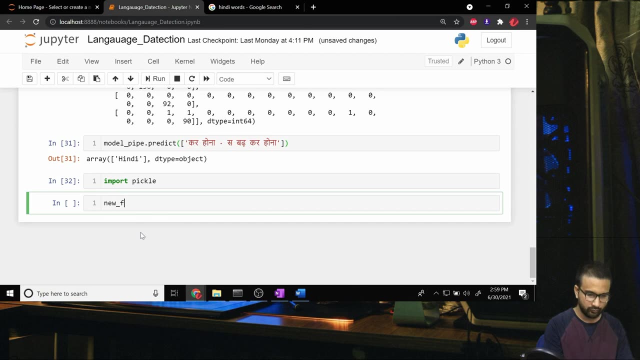 So now we have to save this model as a pickle file, because we want to use this model on our inference And we also want to create a web app out of it. So in the next part, let's import the pickle library, open up a file and writing new file. 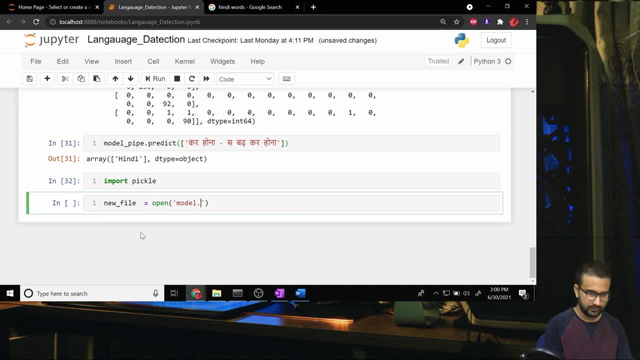 as equal to open. we'll say model dot PKL. Okay, We're going to write this file, So we'll open it in WB mode. This command will open up a file in the current folder where your Jupyter notebook is right now running. 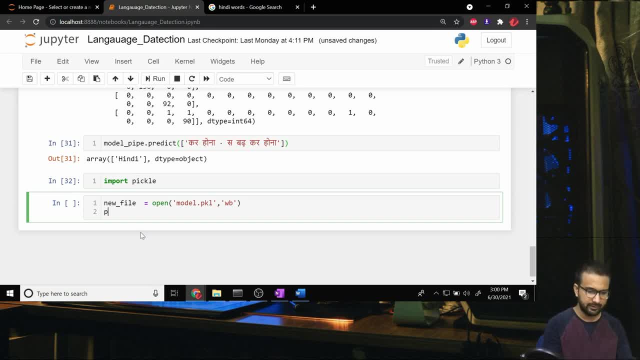 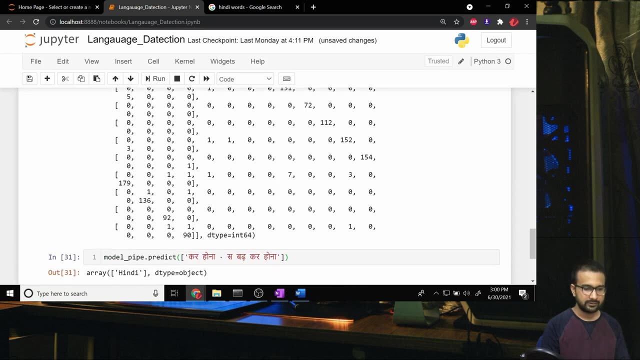 Now, within this file you need to dump your model. So we will use pickle dot dump And if you see you can dump any of the Python object within the pickle file. So you have to give the object name, then the file name. 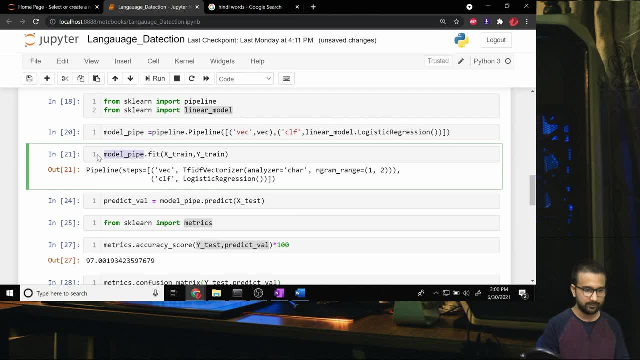 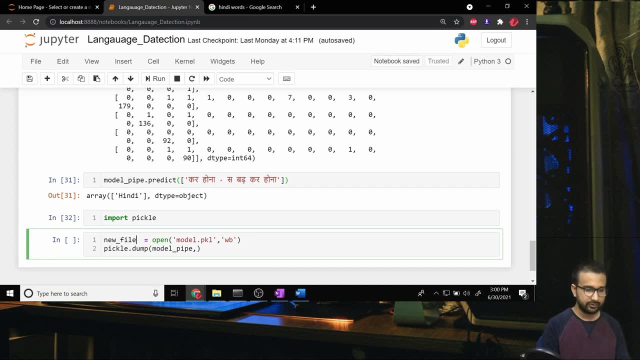 So we have our model saved as in model pipe, So let's save this over here. And then we need to give this new file. Now, this is going to dump your model into this pickle file. At the final we have to close this file. 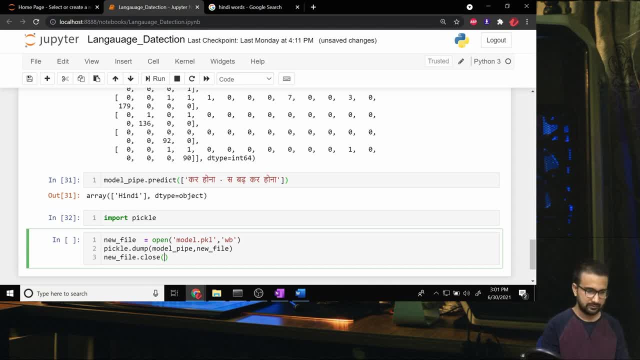 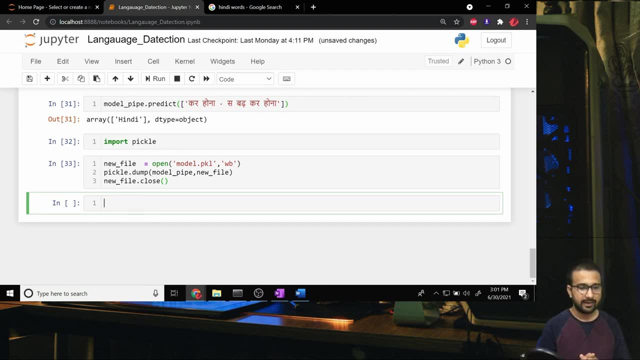 So I'll just write close: Okay, Okay, Okay, Okay, Okay. And you can see this file is now closed and you should have your model ready in the folder where you are running this Jupyter notebook. I can actually check that. 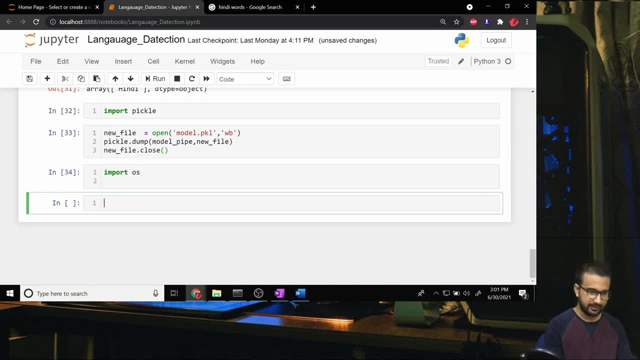 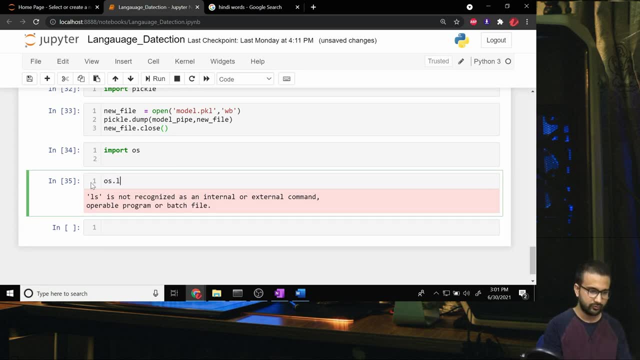 I can do OS- import OS and I can do OS, or I can just do like LS over here- Oh, it's not running- And I can do OS dot list dir. Okay, Okay, Okay, Okay, And here you can see: model dot pickle file is now saved. 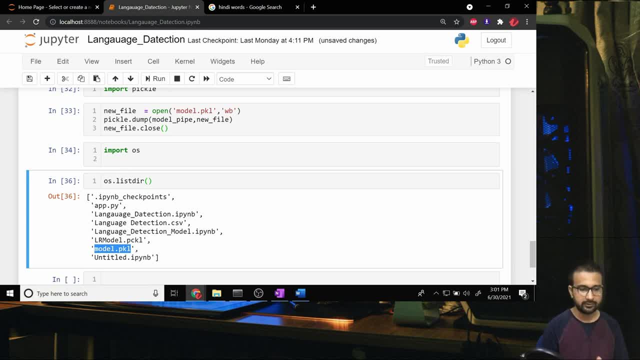 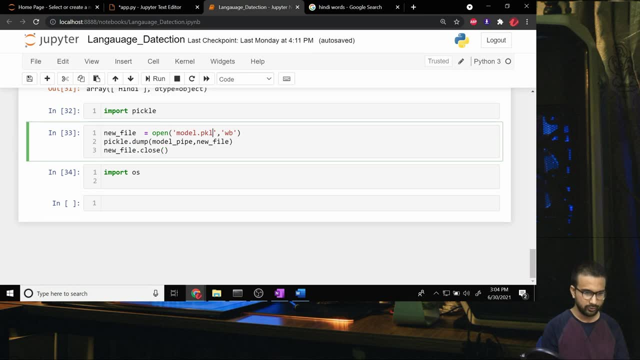 Your model is now wrapped and save as an pickle file in the current folder. So we will use this file again To run the website. If you go to a Jupyter notebook, the format should be PC- KL. I haven't checked it with PKL for me, but I think that's a small mistake you can correct. 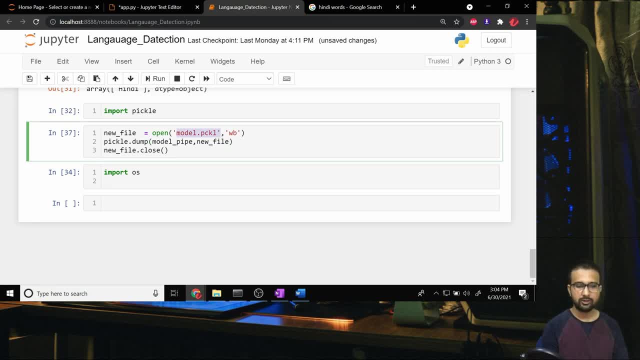 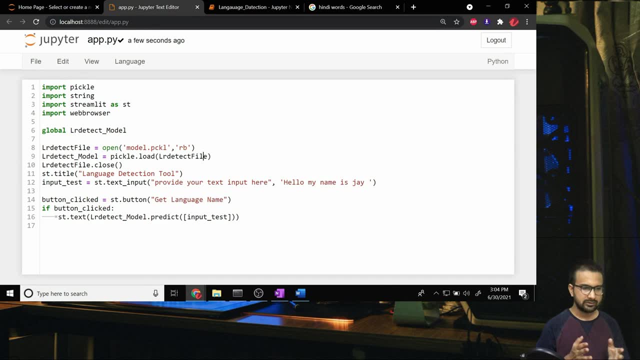 it and run it again. So now you will have this model dot PCL Save within the相信 capital, Okay, the same folder. so if you see the apppy, so this is the apppy that we have created and if you see it's a very small file and this is the file which is creating up that complete web interface. now i 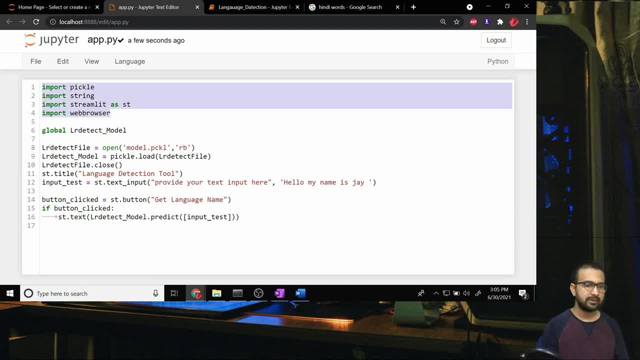 am importing some of the basic libraries- string, streamlight, web browser and all- and then i am having this global variable defined at the start and within this global variable i'm actually opening up that pcl, that pcl file, and then we are loading up the model from that file and we are 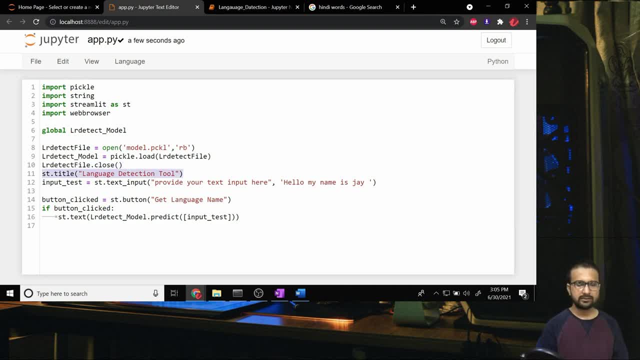 just closing that file. and here, if you see, this is the way how we write code within the streamlit, and you have this sttitle, which will give the title for that web page, and after that you have a input text box and here you have to give the text input so user can give the text input within. 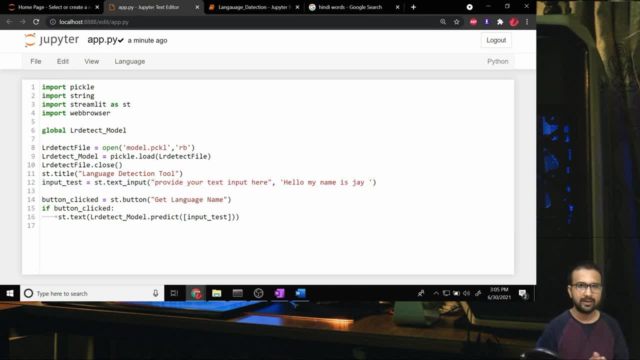 that text box so you can have some default values given to that box and you can have some description for that box. so here i'm writing up the description, that is, provide your text input over here, and then we have the default value that: hello, my name is jay. that is the default value within that app. then we are. 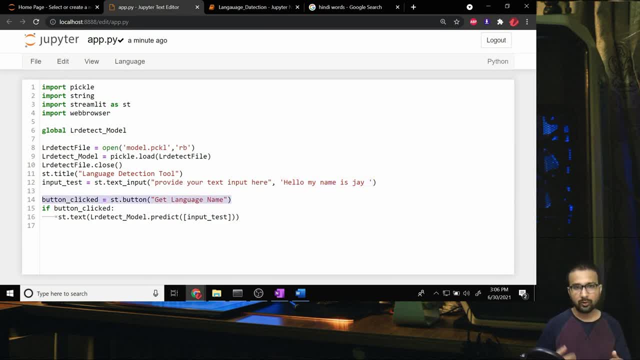 creating up a button by which you will click that button and it will throw out the model output and what it is doing: that all the input given by the user will be saved within this input text variable. and then we are passing out this input text variable within this simple 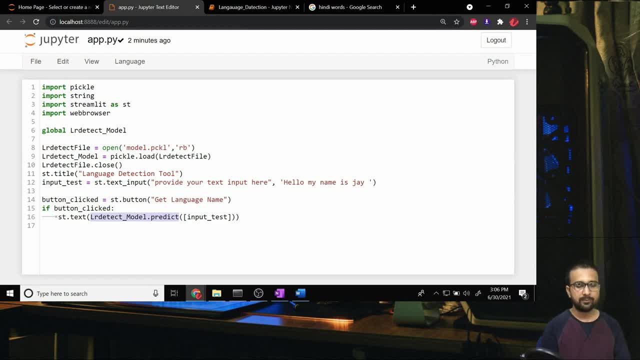 command, and here we are using the modelpredict command and we are passing out that text forwarded from the user site and this will give the predicted label for that input text. now, all in all, we are good with this apppy. make sure that you have installed streamlit before moving ahead and 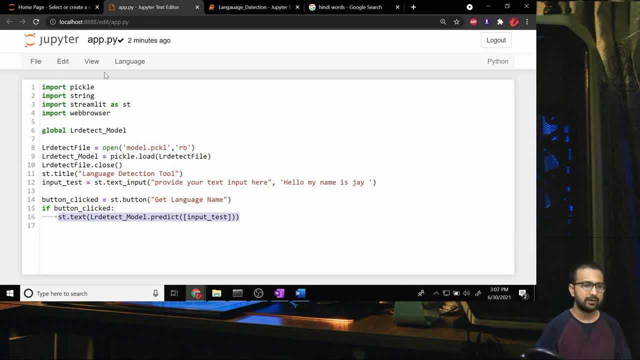 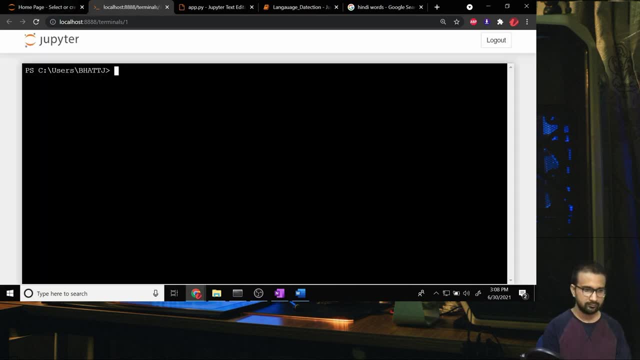 once you have installed streamlit, it's very, very straightforward. i can actually go back over here. i can go to the terminal here. so once you will be in this terminal, you need to do streamlit run app dot py. so, as you can see, i have just given streamlit run apppy, so right now i am doing this colon dot.